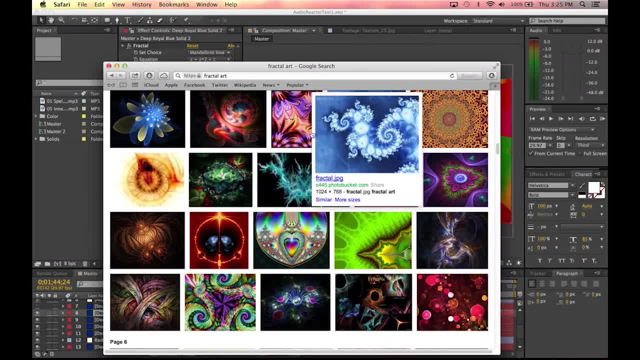 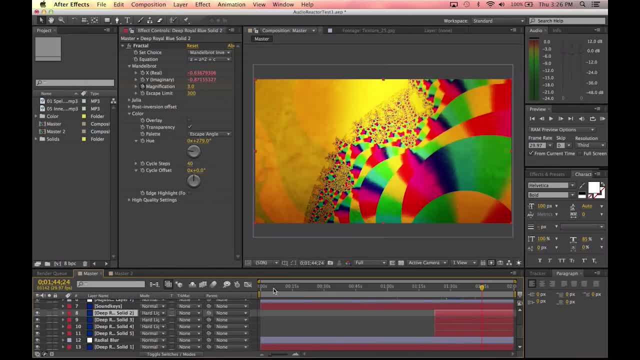 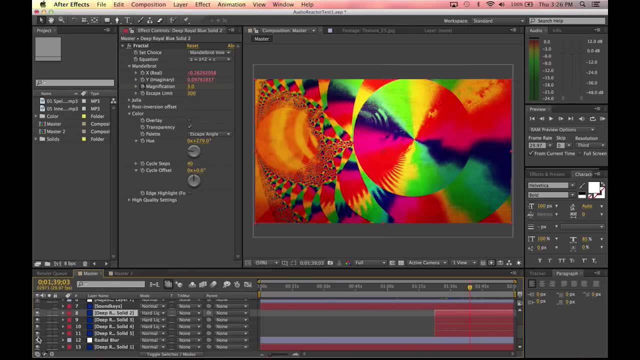 You can see they're all the same shape And they're repeating in the shape of the same shape. So very interesting stuff. All right, So over here in After Effects, you can see my original composition here, If it'll load. Yeah, Okay, So there's actually five different. 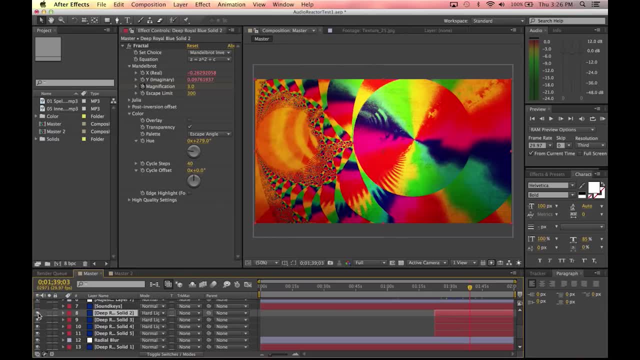 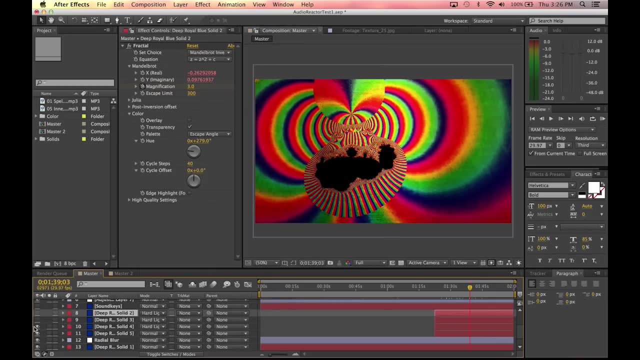 fractals here And I layered them over with hard light. So here's the first layer gone. Second layer: you can see all the banding here. I'll show you how to do the colors. Fourth layer: I guess that one was off screen And that's another fractal, So let's up and 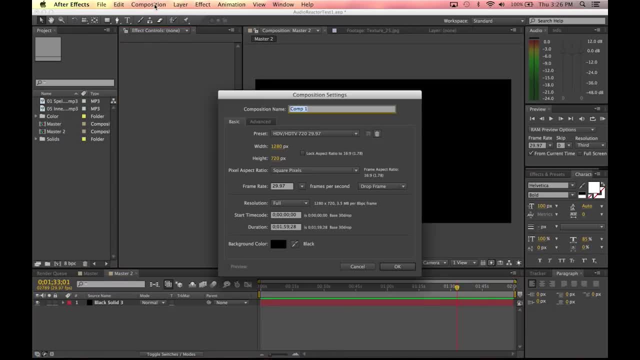 do a new composition here. Let's do composition, new composition. Okay, We're going to call this Tutorial Master. We'll make it 1280 by 720.. That's HD, And duration doesn't really matter. Okay, So here we are. 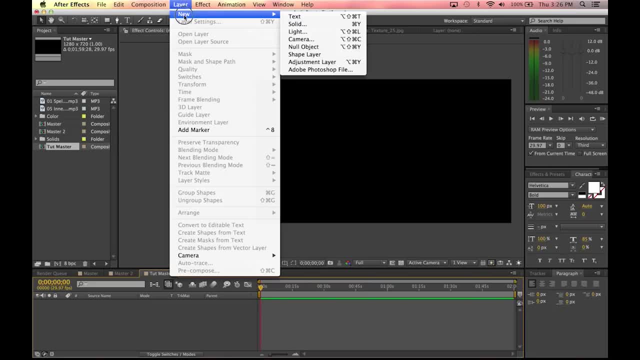 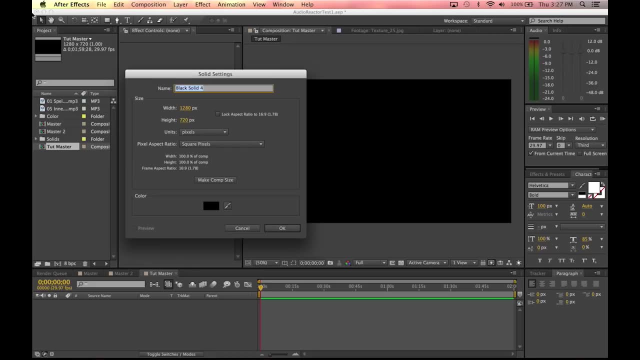 We got our beautiful blank composition. Now I'll do layer new solid and make comp size. if it's not already, We'll just call this fractal 1, just so we don't forget: Color doesn't matter, because we're going to go to effect. 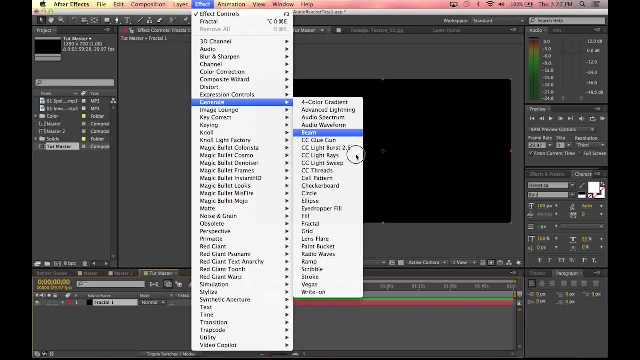 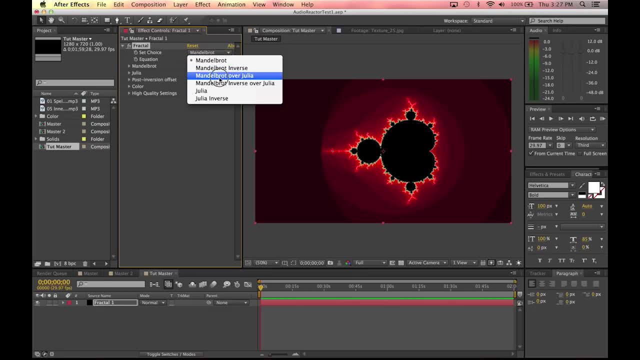 Make sure the layer is selected, Generate Fractal And we're done. No, I'm just kidding. Here's the type of fractal we have here, And I guess this doesn't really matter too much. It just depends on the look you're going for. 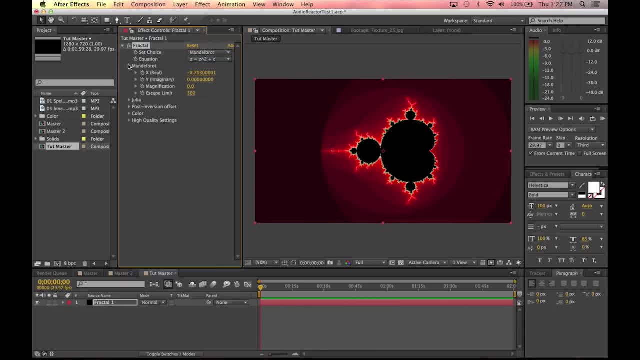 I personally like the Mandelbrot. So you can see as we move through the timeline here, nothing's happening And that's because we have nothing animated. Let me just scroll through these properties here. So this is the X real value. 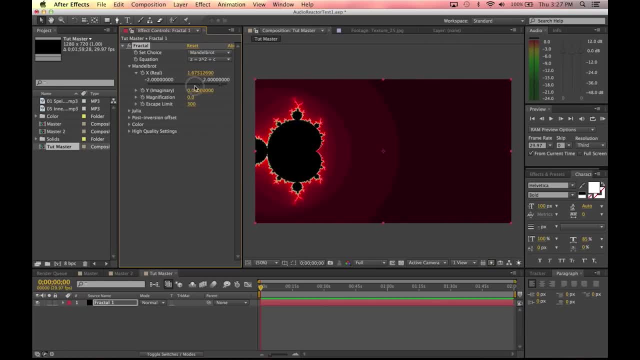 It's basically like scrolling across the scene in X space on the X axis- And this is for the Y axis, up and down. And here's the magnification, So you can basically just scale into this whole thing. Wow, It goes really fast. 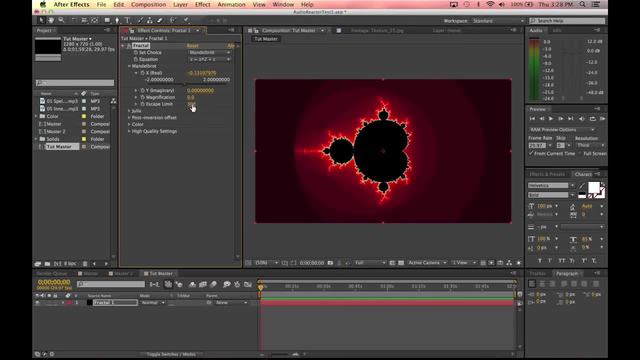 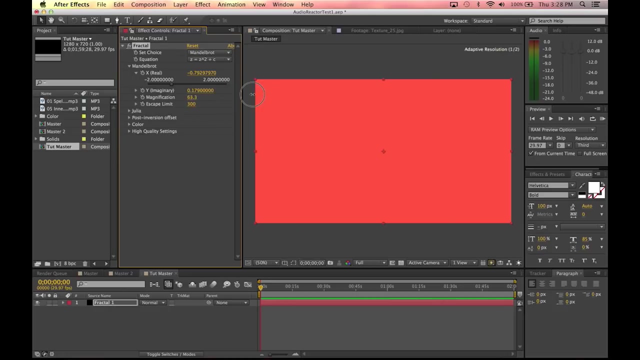 Yeah, Now the escape limit is something interesting Here. let me see if I can zoom in here to a part where you can see, All right, And we'll increase the magnification here, So you can see there's tiny, tiny, tiny, tiny, tiny, tiny, tiny fractals here. 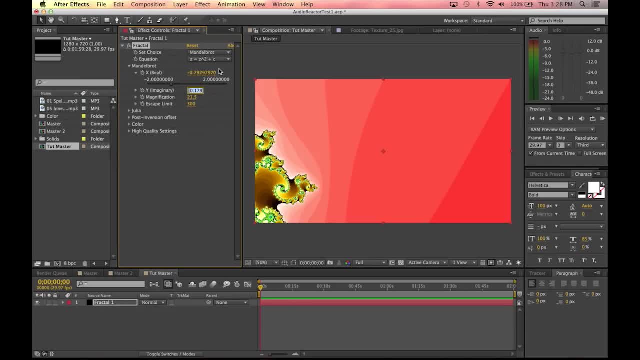 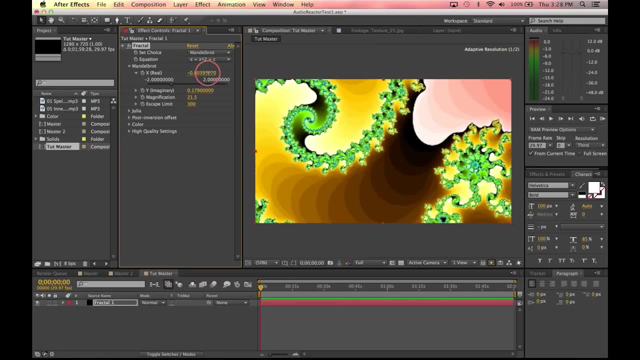 And whoa, I'm going to move really slow here. I'm scrolling by really small values by holding down Command on a Mac, I'm not sure what it is on a PC. I'm scrolling here and it goes really small instead of bigger numbers. 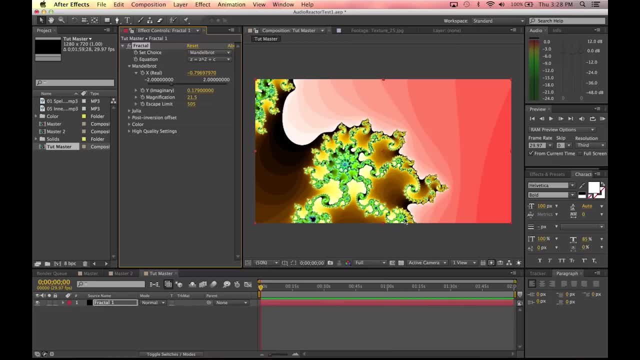 Now, if we increase the escape limit, it'll actually add fractals. You probably can't see that, But it's adding more fractals down here. So if we start Decreasing this, it's decreasing the number of iterations of fractals. 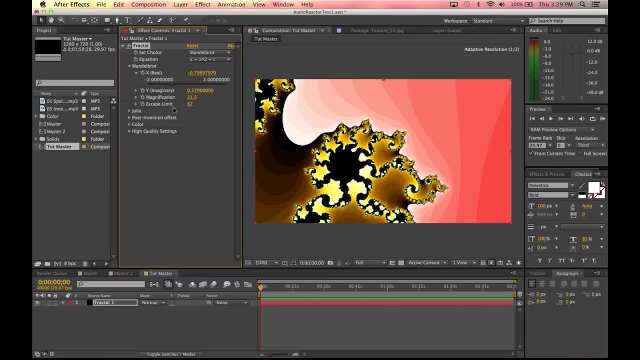 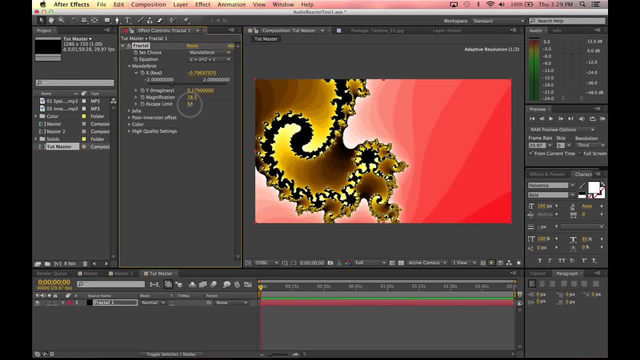 So you can see here: some of them disappeared. decrease it. some more, even more disappeared. It's basically just stopping the fractal because I mean it's not infinite on a computer, Otherwise you'd be rendering for an infinite amount of time. 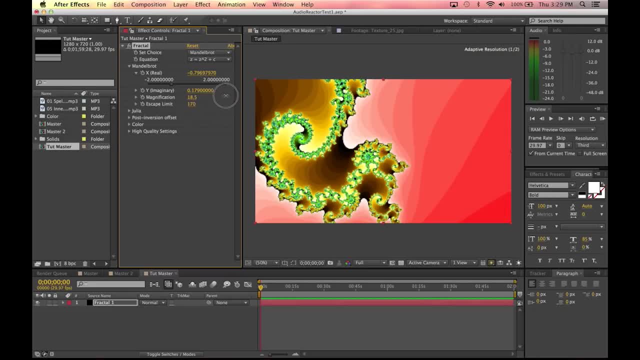 So I find that about 150 is okay. You can get a lot of detail in with 150.. So, and you don't need to waste Processing power by going to 300. But if you want to go for it, I guess now we're going to let me. 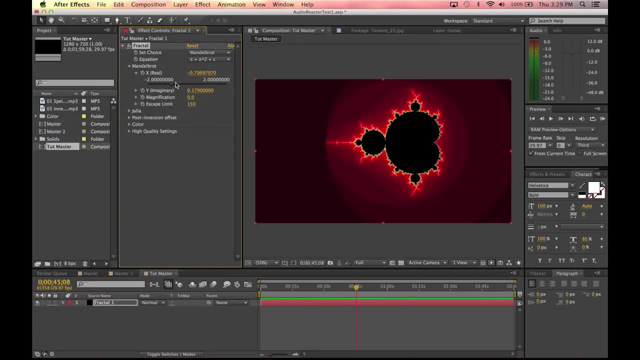 Oh, that was the dog. Let me do zero magnification so we can see everything here. I'm going to reset these values by. you can right click on it and do reset. Right click reset. just to make sure. the fractals in the center here. 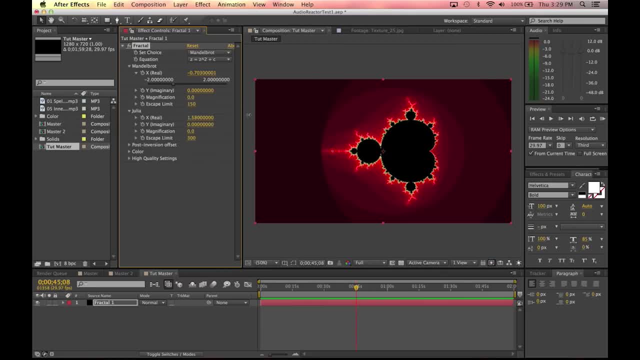 So oh, and the Julia factor. I'm actually not 100% sure what the Julia factor is. I I didn't really use it in mind, So I guess I'll do a little research after this tutorial and might post it below. 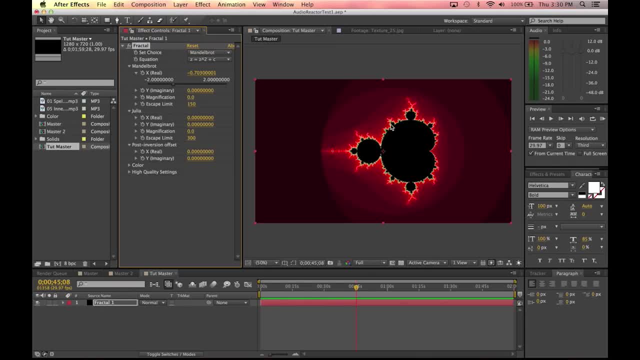 I think it's actually another layer of fractals that kind of creates the indents. But I could be wrong, post inversion off, So you don't need to worry about that. Here's the color settings. So I had it set to, I think, escape angle on one of them. 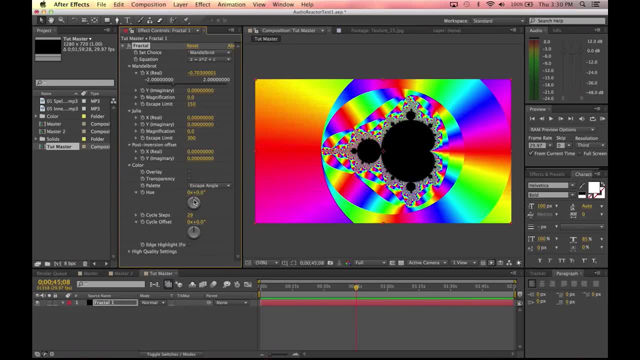 Yeah, that creates a really strange, really strange properties. here You can change the hue and kind of Offset that. You can animate that even if you want. Here's the number of iterations and you can offset that to creates a little bit more banding though. 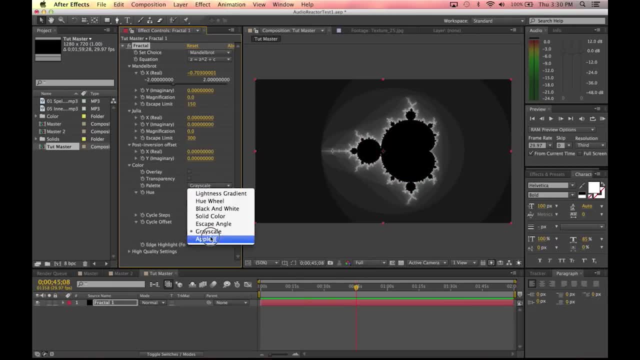 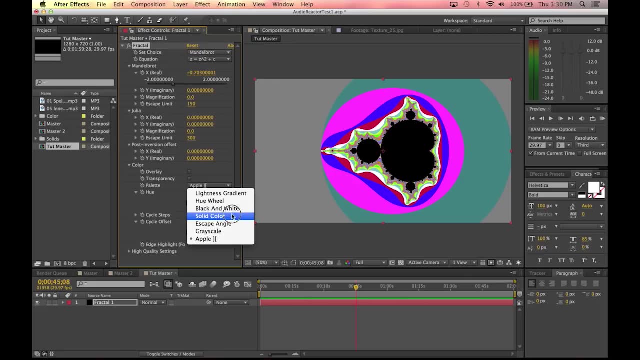 So I don't know, Just depends what effect you're going for. I mean, I kind of like this one. It's kind of cool, And of course you can change the hue on all this. Oh, I guess you can on that one. 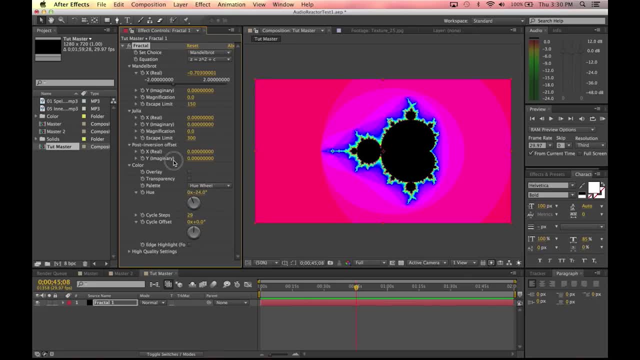 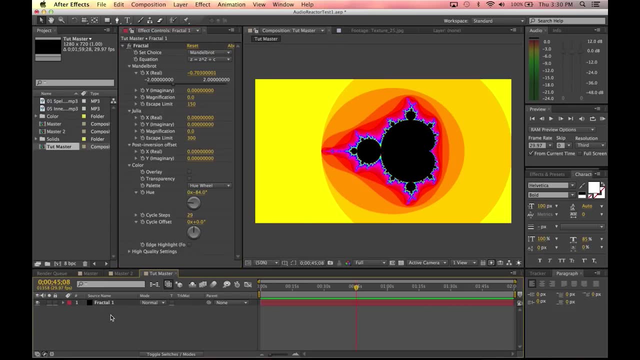 Oh, there we go. You can change the hue on that one, So I mean you can do all sorts of stuff And that's That's kind of cool, Going from red to yellow. Yeah, I guess we'll keep that. 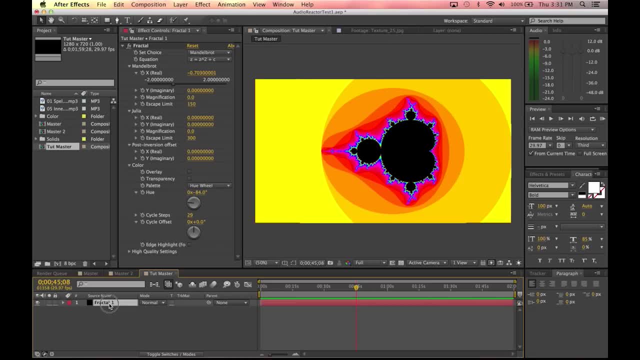 OK, so that's our first fractal And actually I guess we should animate it. So here I'm going to alt click on this keyframe. Now, this is really important. I use this a lot, this expression, So I'm just clicking in this expression area here under that value that we just keyframed. 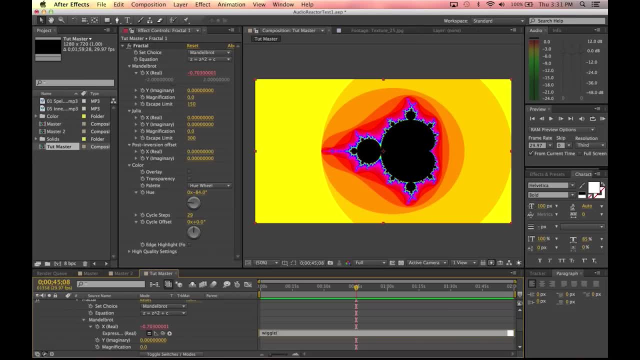 Going to type wiggle and parentheses. I think I did 0.1 or 0.25.. And that's the number of iterations per second. So it's going to cycle through this value 0.25 times per second comma. 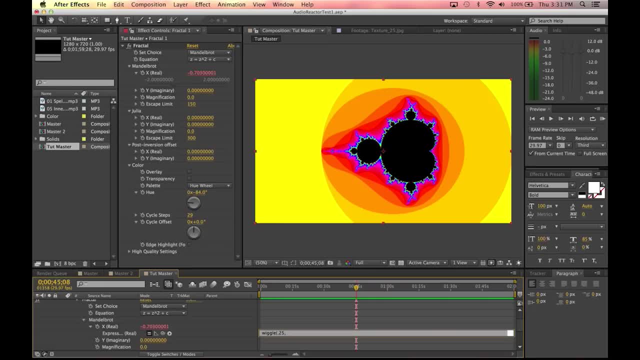 And this is our value, that it's going to cycle through, And I think I did, let's do 500 pixels, And so it's going to fluctuate this value by 500, 0.25 times a second. So OK, 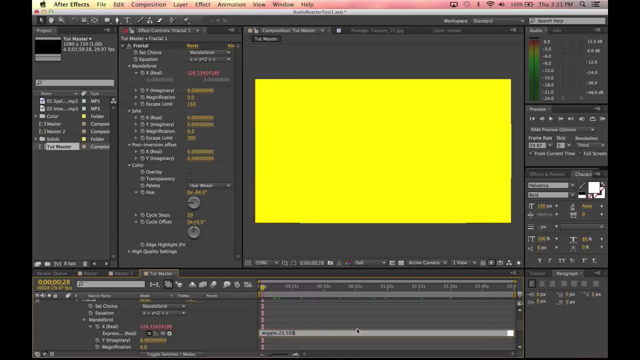 Oh, that was way too much. Let's go 2.. There we go, All right, So now it's moving back and forth. Yep, Here, let me hop back into this composition and I'll see what values I used. 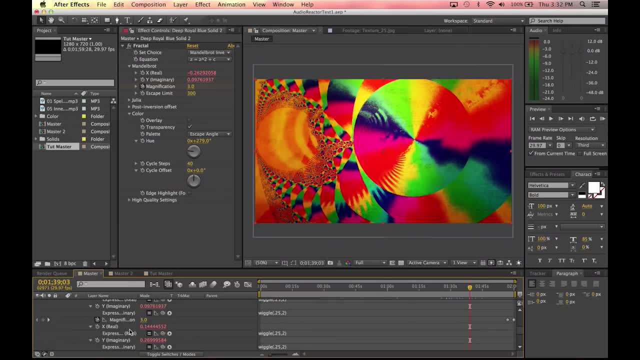 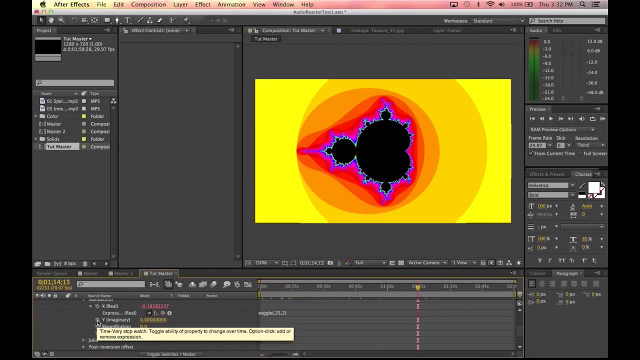 Yeah, 0.25 to 0.25 to yep. OK, So now we're going to keyframe the y value. You can do it here Or if you click on the fractal. again you can, OK. 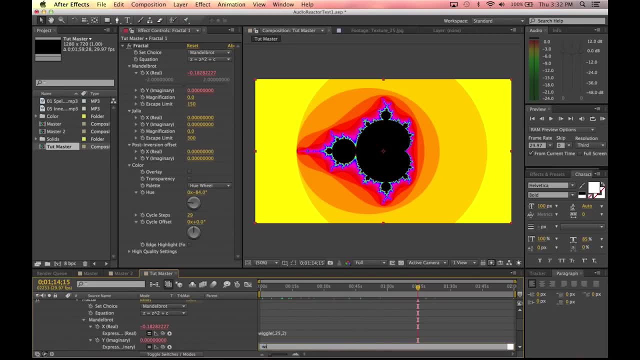 Alt-click up here We're going to enter the same value, wiggle 0.25 comma 2.. So it's 0.25 times per second. It's going to fluctuate by the value of 2.. Sorry, not 2 pixels. 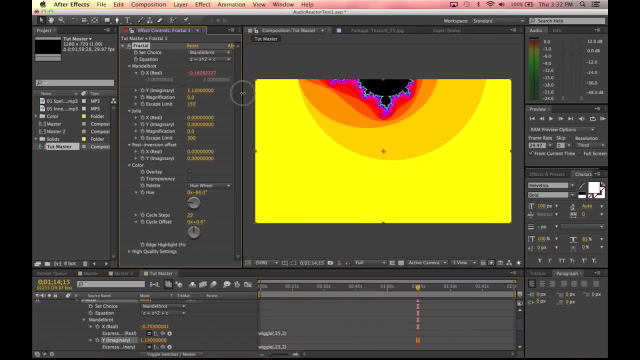 The value of 2 on the slider, which I mean you can tell 2 pixels is, or 2 on this value is going to move quite a bit. So 500 was way overkill, So yeah, So that means that it's going to move in x and y space randomly. 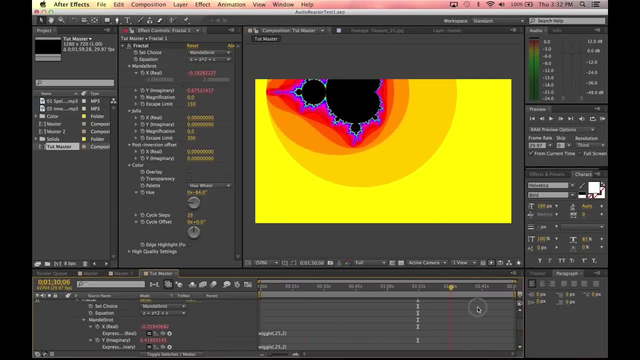 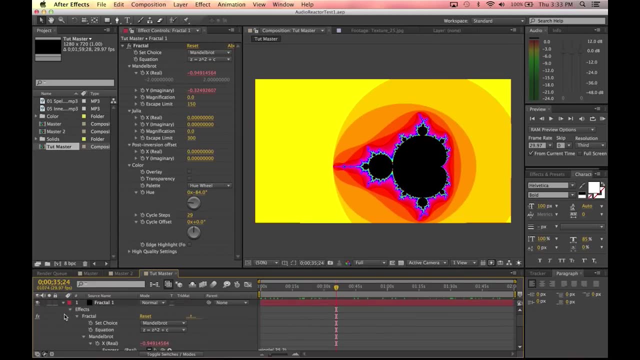 It's going to move in x and y space randomly throughout this entire time. Not too exciting. you think It's just a little fractal bouncing around on screen. But once you start layering fractals on top of each other, then things can get interesting. 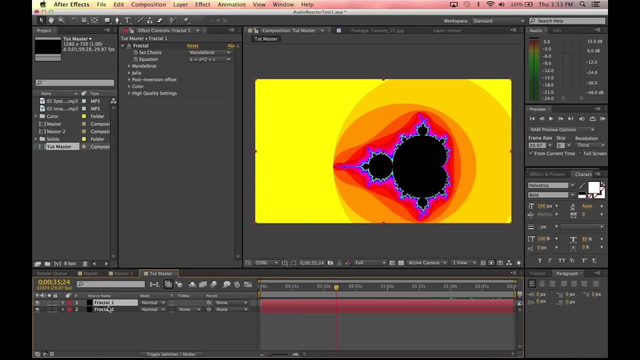 So we're going to duplicate this. We're going to call this. I did that by pressing Command D on a Mac. I'm going to click that layer, press Enter. I'm going to call it fractal 2, just so we don't get confused. 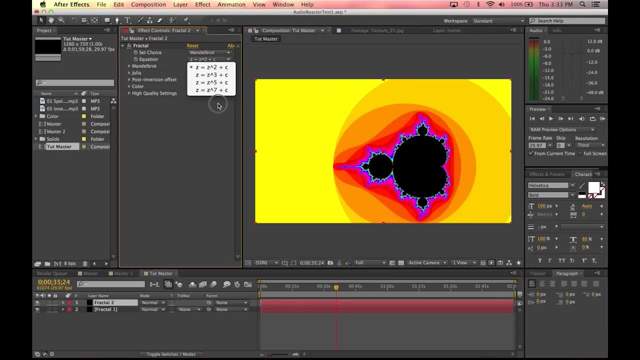 You can even change the type of fractal here. You can even change your equivalent. OK Equation, Let's do that. Yeah, There we go. It kind of looks like a snowflake. All right, We're going to change the color. 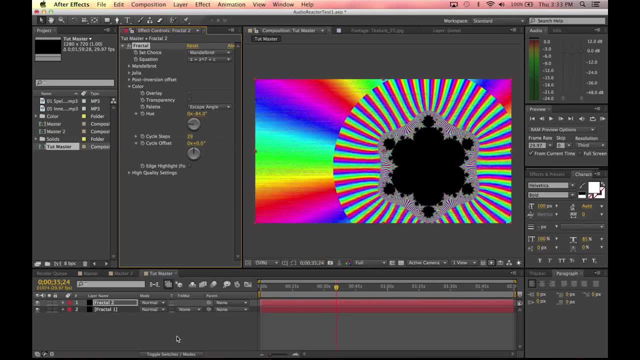 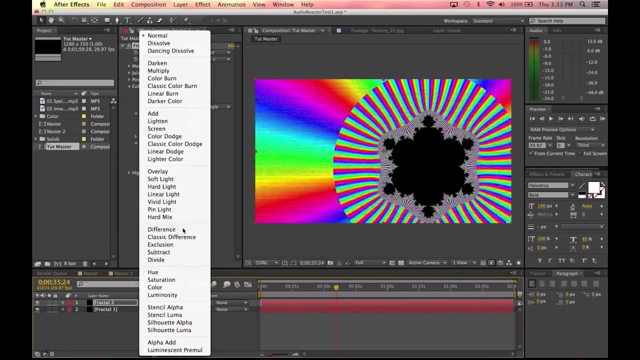 Going to make this escape angle. Yeah, That's cool. All right, Now this is where it starts getting cool. You do Mode And you can experiment with all sorts of things. I tried a lot of stuff. Difference gets you some really cool effects. 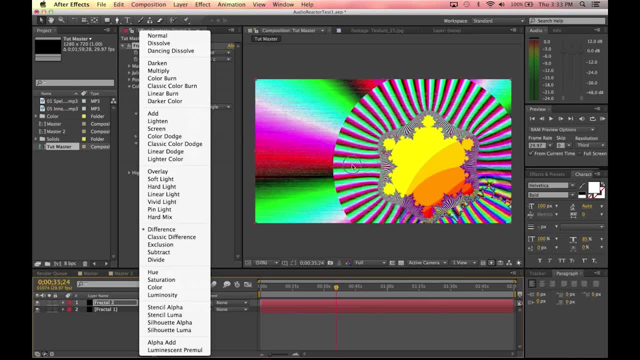 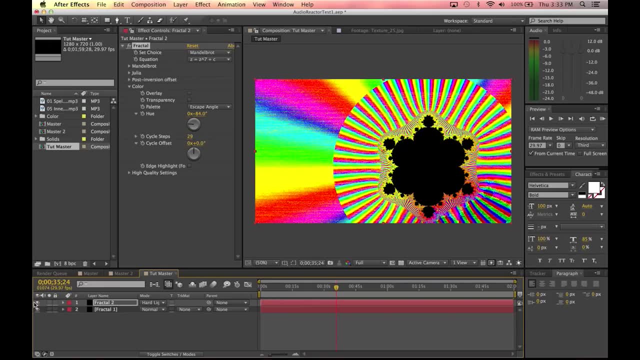 But it kind of makes this whole thing hard to get the right color that you want in there. So I used hard light just to kind of preserve the colors a little bit. So you can see this is with the fractal and this is without. 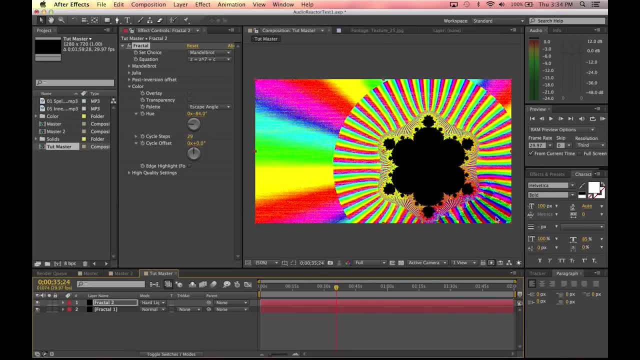 You can see that fractal there. So basically, what's going to happen is, when this fractal moves into this black area, then it's going to start showing up. So in fact we might- if we scroll through, we might be able to see that. 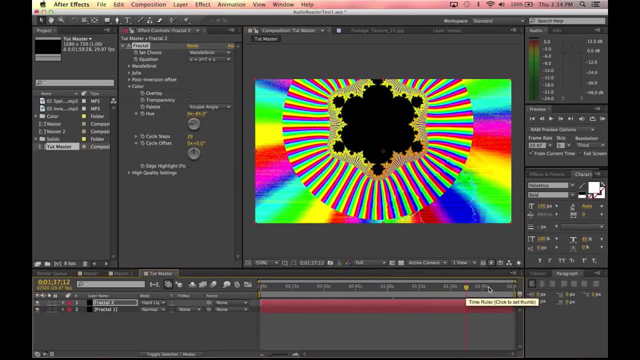 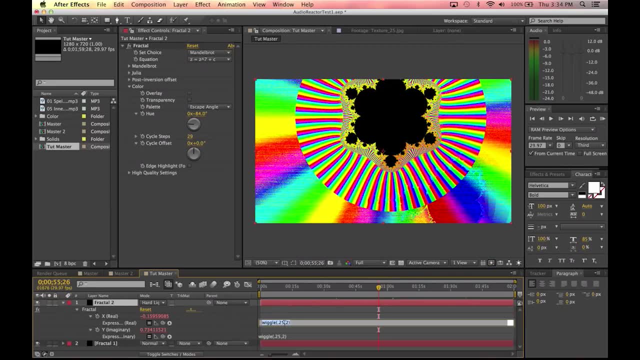 Yeah, OK, I don't really see that happening, But let's OK, All right, So I'm going to change these values a little bit, So just press U to reveal the key frames. here I'm going to go to 3.. 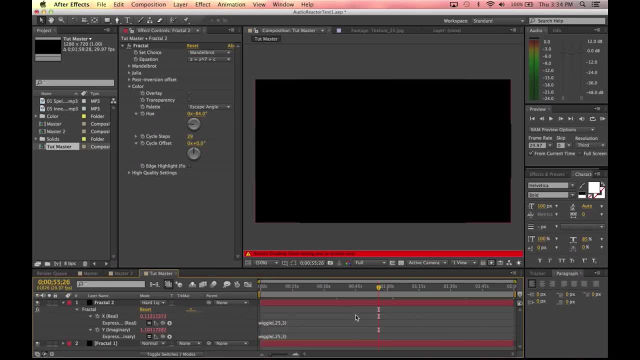 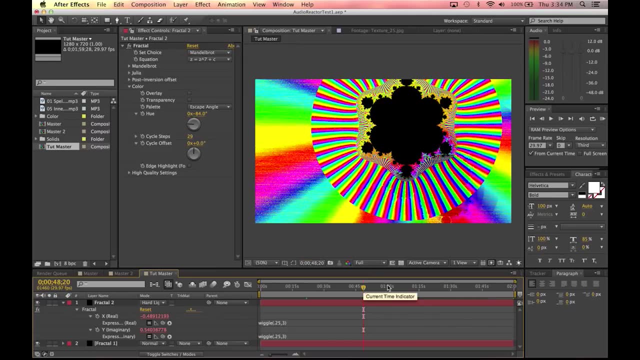 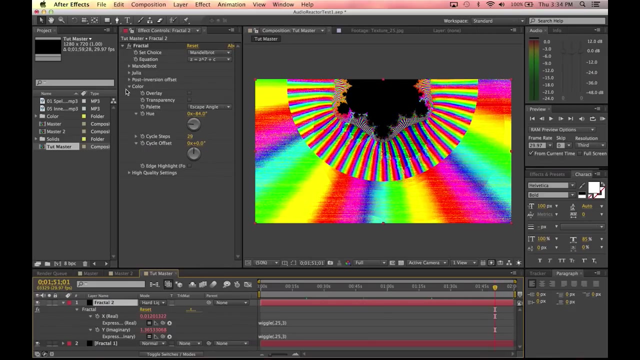 3 here. All right, Might just have some refreshing errors, So, all right, I'm going to click on this fractal. We're going to go to Mandelbrot, OK, And increase the magnification, And this is going to give us some really interesting stuff. 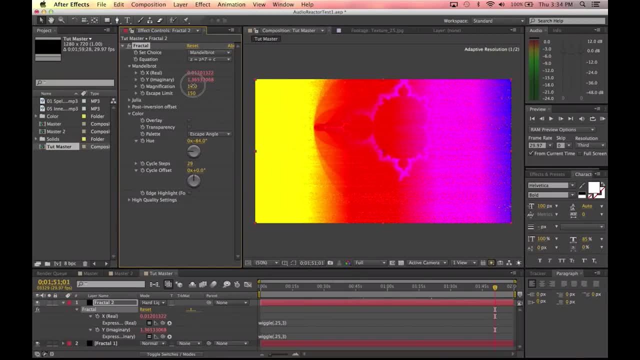 All right, So you can see all sorts of interesting things are happening here. Yeah, Here's the edge of the fractal, which I really like. It's kind of revealing the fractal underneath here. If we set it to difference it might. 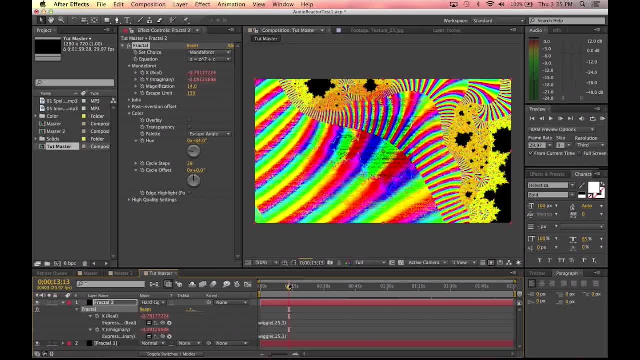 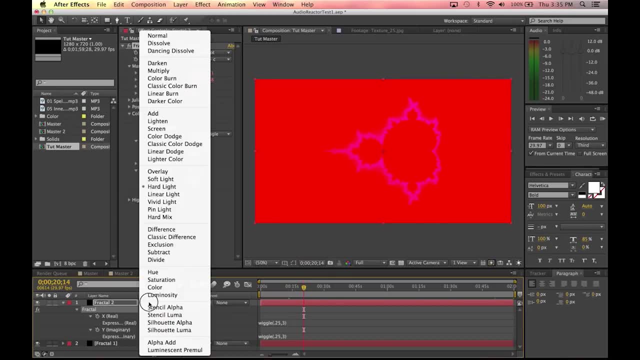 Yeah, There we go. I guess I'll set it to difference for this, Maybe not Hard light. Yeah, OK, All right. All right, So I'm going to go ahead and do this. I'm going to go ahead and do this. 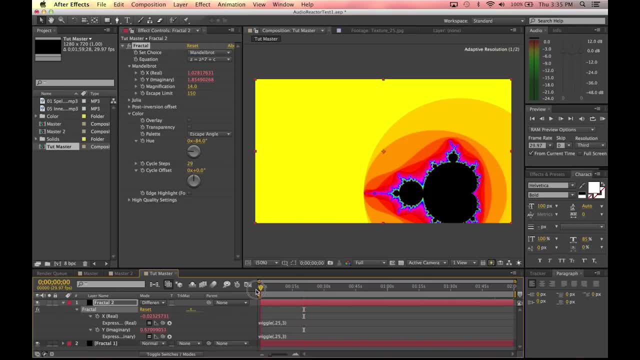 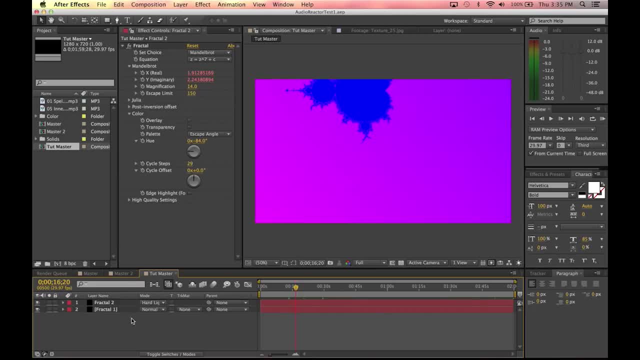 And really I mean because of the random movement. you're going to need a lot of fractals, which means it's going to be really hard on your computer rendering these. So make sure you set aside an ample amount of time to render. 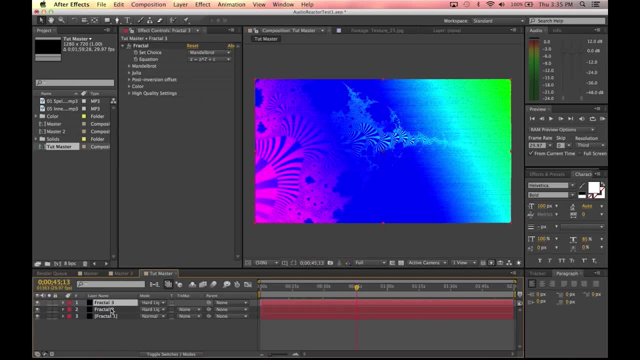 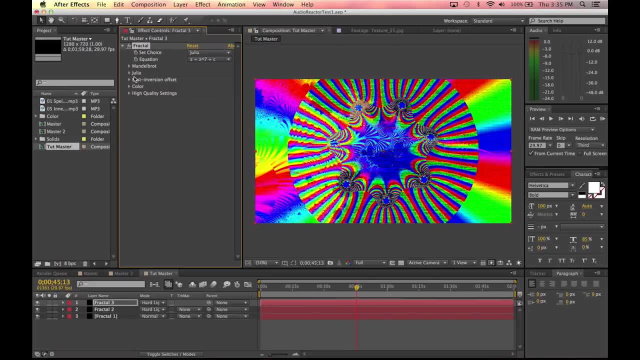 All right, Now we're going to duplicate this layer again. Command D: We're going to change this fractal. Let's use Julia. Yeah, Oh, that's strange, All right, All right, All right Color. I love fractals. 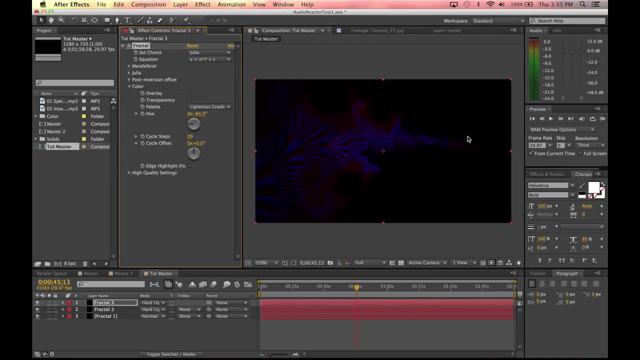 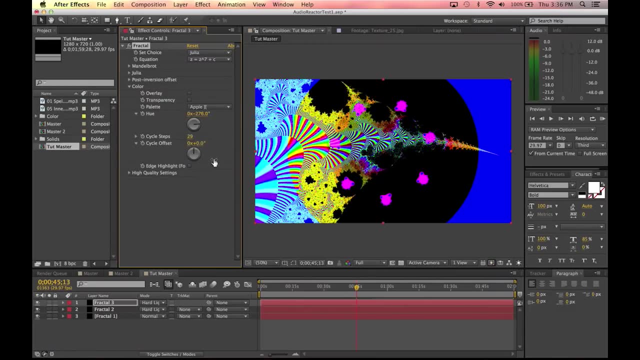 You get something different every time. Here's: Oh, that's interesting. I don't know if you guys can see that It's real dark, but I kind of like that effect. Yeah, But I'm going to. Let's go with apple here. 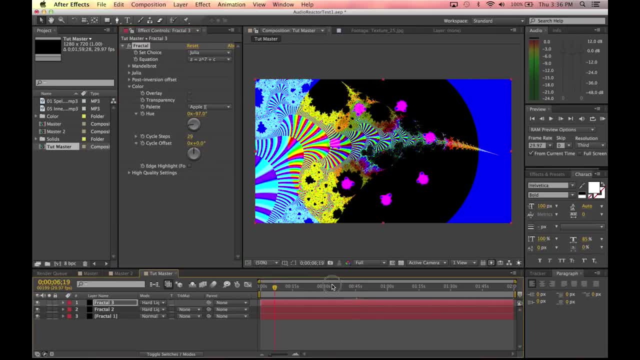 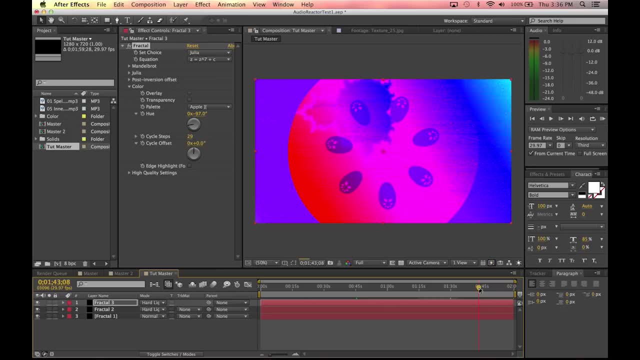 Yeah, OK, So I like that Kind of scroll through and see the effects. It's real slow on rendering. It's rendering three almost infinite Equations at the same time, so that's why You can see it's moving quite a bit here and changing a lot, which is great. 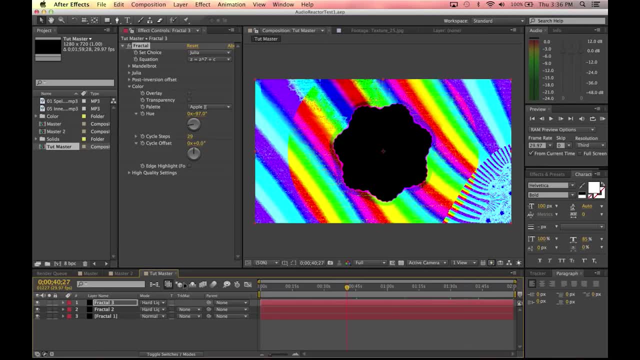 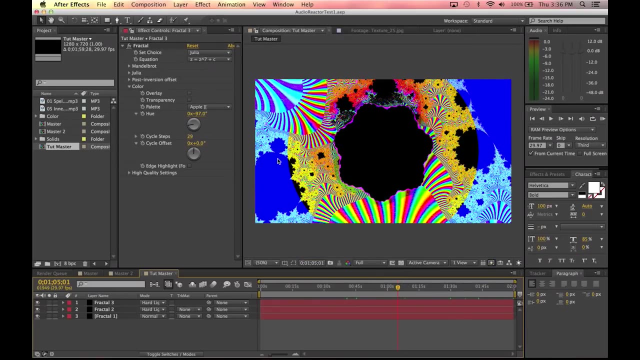 We want it to be really dynamic And I'm sure if you experiment with, I know, Video Copilot has this plug-in called Spin, I think it is. It came with the Evolution Pack and it creates symmetry. It kind of duplicates this layer and spins it, creating some kind of 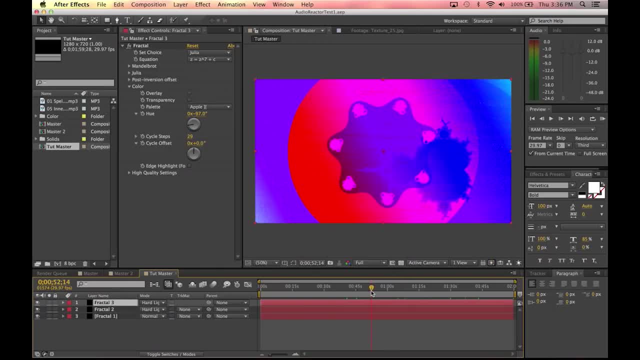 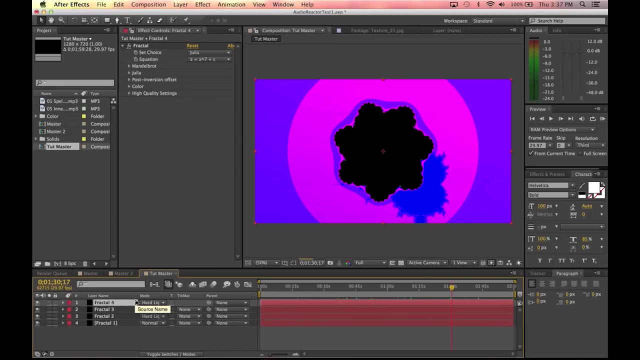 Kaleidoscope effect. I imagine if somebody were to go through this tutorial and use that, you could get some really interesting results. I almost did that, but I didn't, So if somebody does, please show me. All right, I'm going to duplicate this layer again. 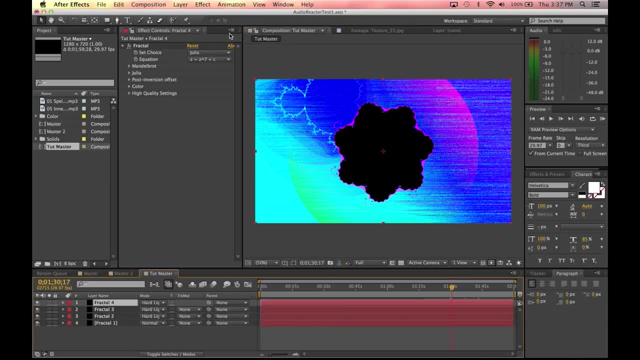 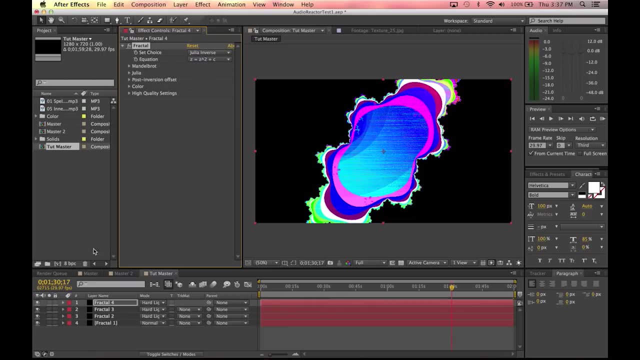 You can see, we get a completely different effect. now I'm going to call this Julia Inverse, Change it to a different equation, And really this doesn't matter. You guys can do whatever you want on this. So yeah, here's. 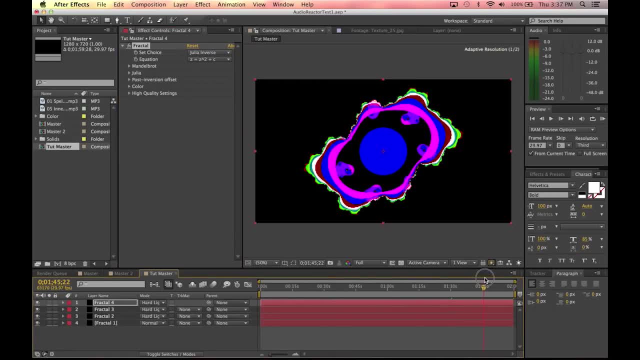 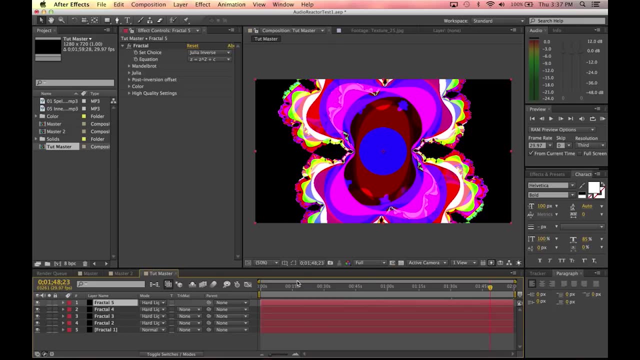 Gosh, another interesting effect. Wow, I like that a lot actually. Okay, We're going to duplicate it one more time. I mean, you guys can do this as many times or as few times as you want, You don't have to follow exactly. 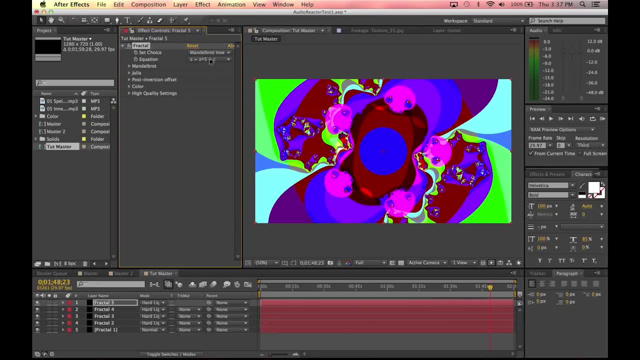 In fact, I recommend that you don't, because you'll learn more. Let's do Mandelbrot. Mandelbrot over Julia, maybe? All right, We're going to scale our scheme here to escape angle. Ooh no, 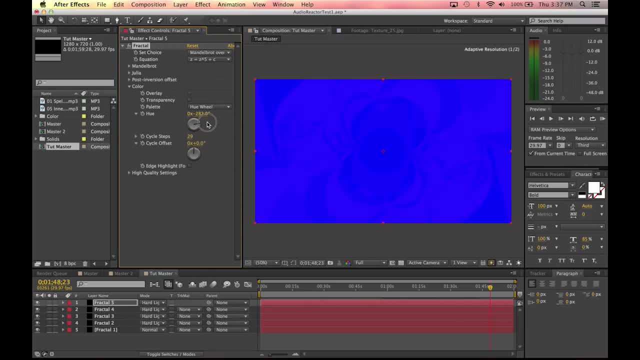 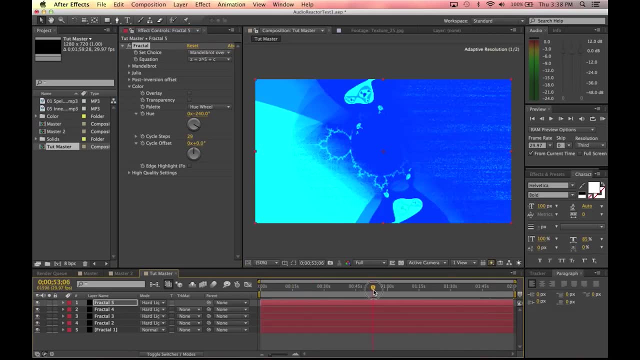 That's real bright Hue wheel maybe. All right, I'm just offsetting that hue. Yeah, I don't know about that. I think it might be too big. so I'm going to go to Mandelbrot. We're going to scale down. 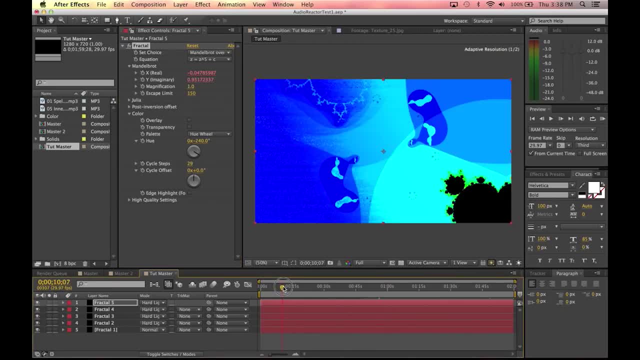 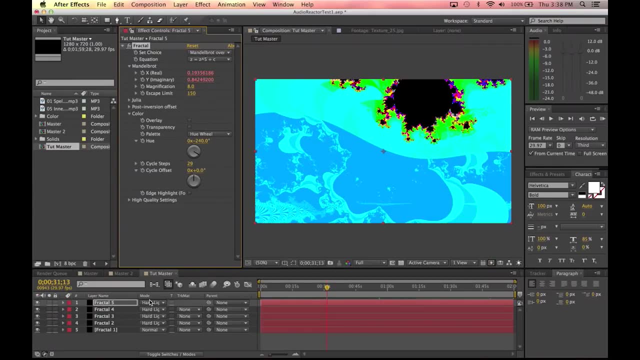 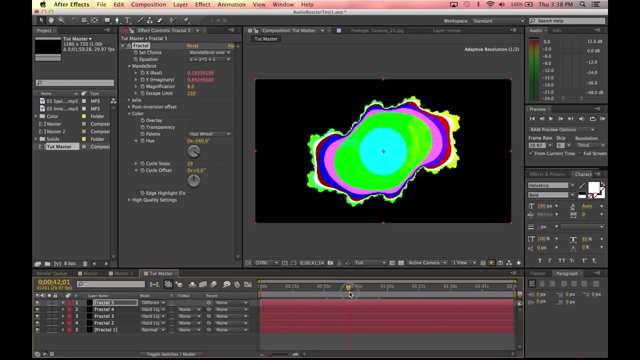 That's why It was basically tinting the entire scene blue. So I'm going to scale down the thing here. Actually, let's scale it up. Maybe change the overlay mode to difference. All right, Sure, Okay, Here we go. 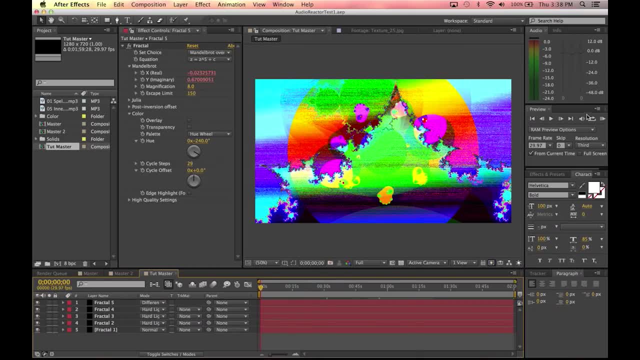 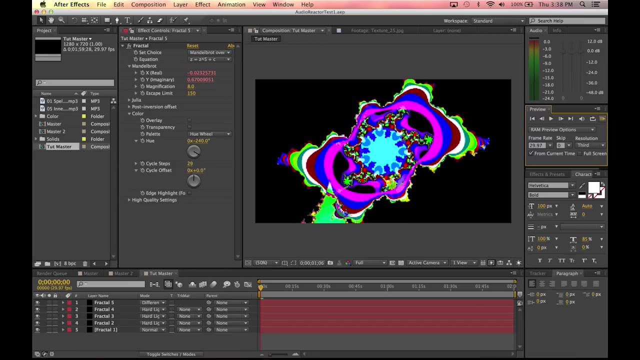 So I mean there's our fractal animation. Let me just do a quick RAM preview here. Third resolution, Because it's going to take a long time to render. All right, So you can see everything is changing here And you get some really cool effects. 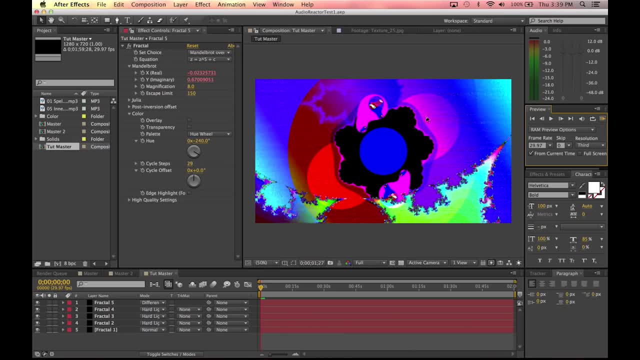 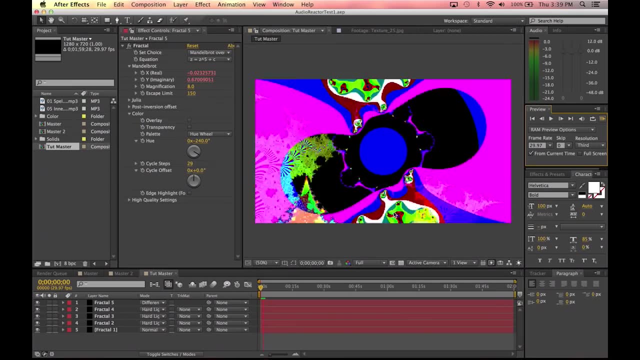 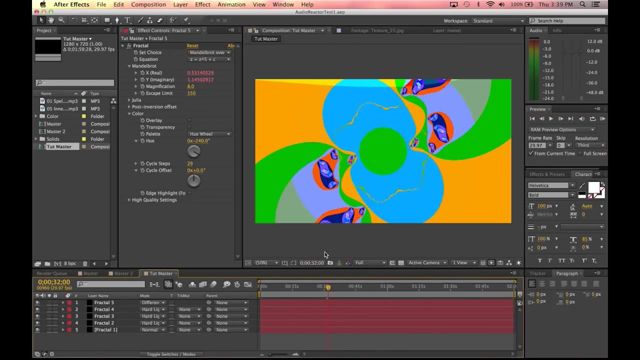 Stuff zooming in and out, and, yeah, I like it a lot. So there's our fractal animation, Yep, And what I did just to make it a little bit more interesting was I took some textures, And this is from a video: copilot pack. 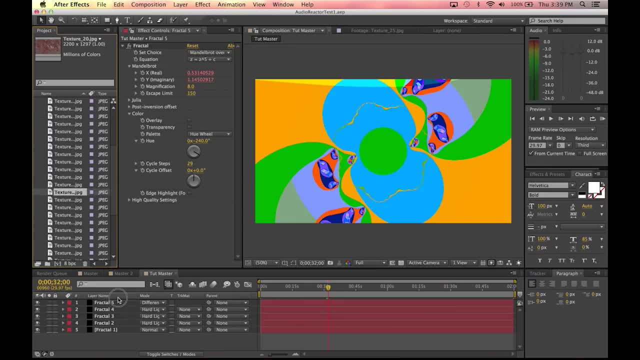 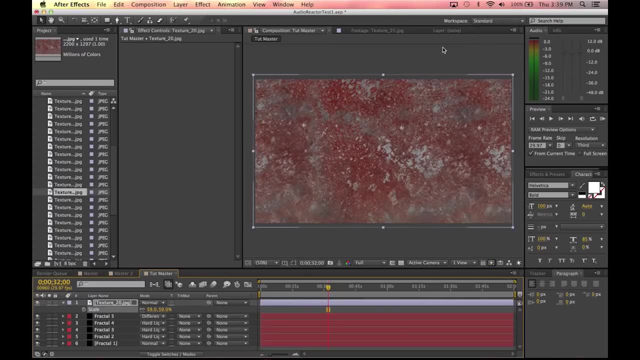 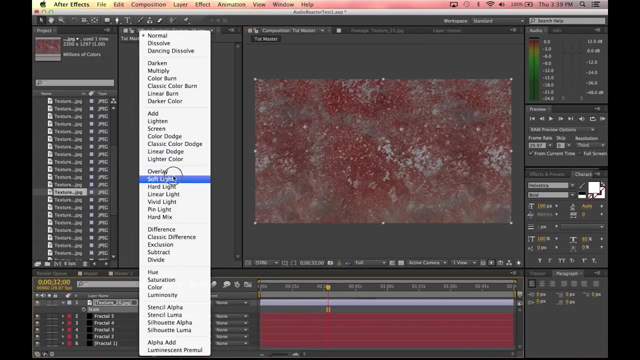 But you guys can use whatever you want, Just pulling some textures from the internet, Yep, And just scale them down, Make sure they fit your composition. You can actually do transform fit to comp Love that. Change the mode to let's do overlay. 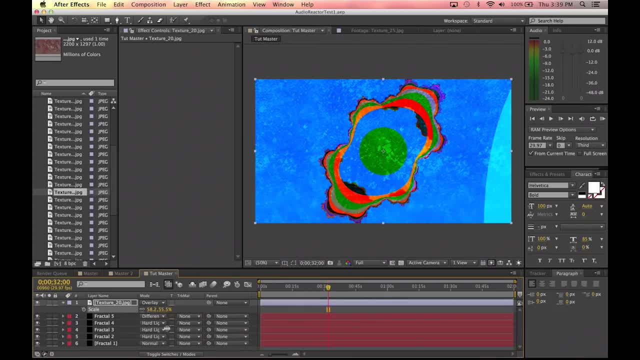 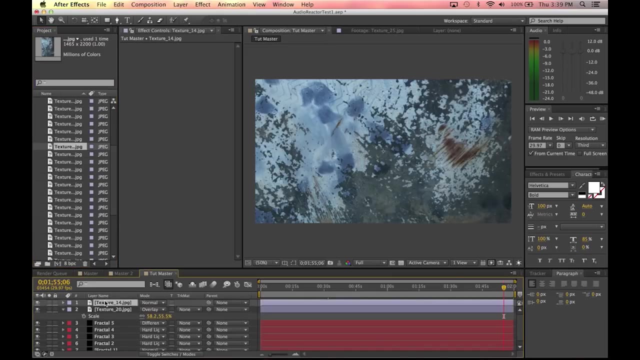 Yep. So here's some little texture in the background. I like it. It's going to change with the colors And pull in another texture. This is a really interesting effect that I kind of learned just by experimenting, Going to rotate it so it fits in. 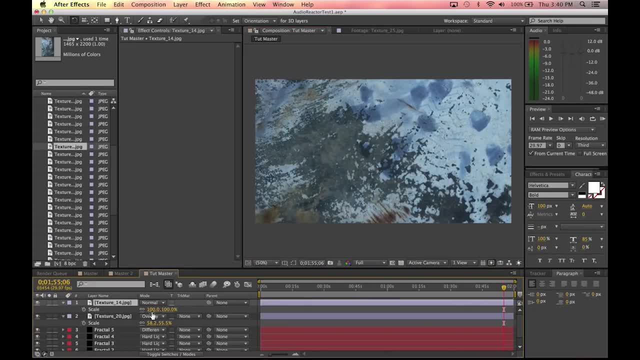 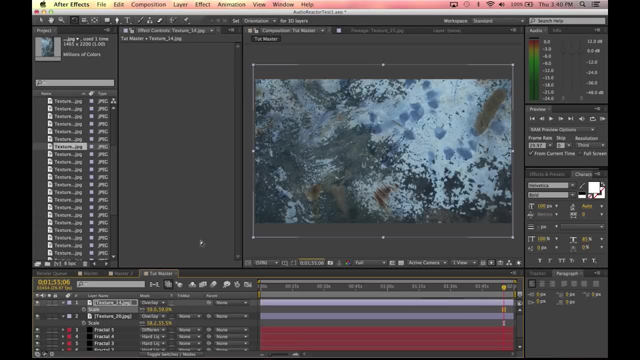 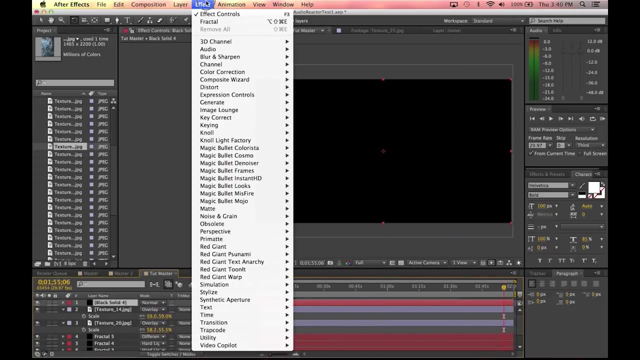 I'm going to go to scale this down. There you go, So it covers the whole comp. We'll do overlay again. Now here's an interesting effect: If you go to layer new solid, You go to- I think it's effect noise and grain fractal noise. 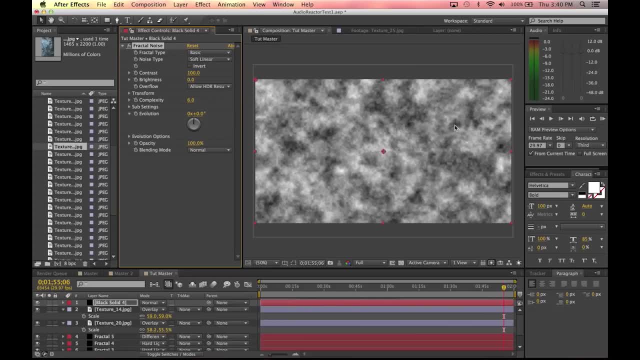 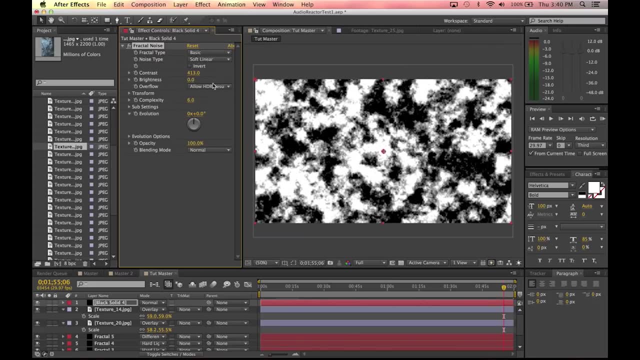 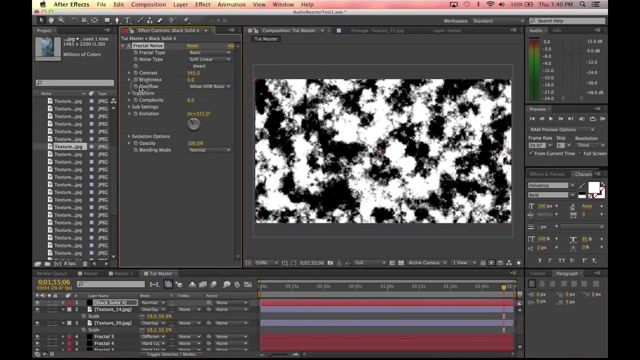 Another use of fractals. Now you can see, this generates some white and black values, And we can change these values and make it whatever we want. Increase the contrast here so you get almost just white and black And you can animate the evolution. 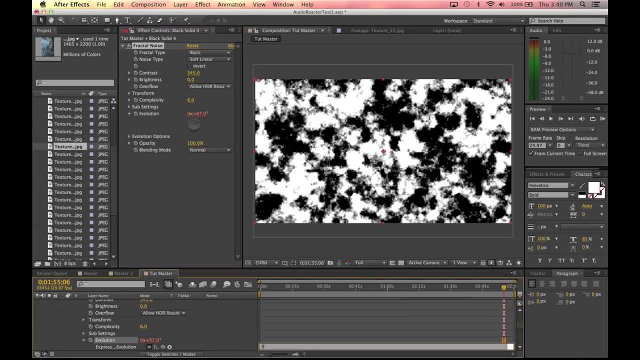 So I'm going to alt click on this evolution. I'm going to go to time And time- this is a little asterisk here- 20.. So it's going to take the time value, multiply it by 20. And that's going to be our evolution. 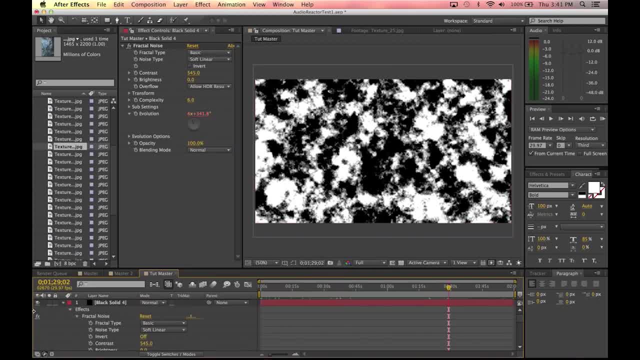 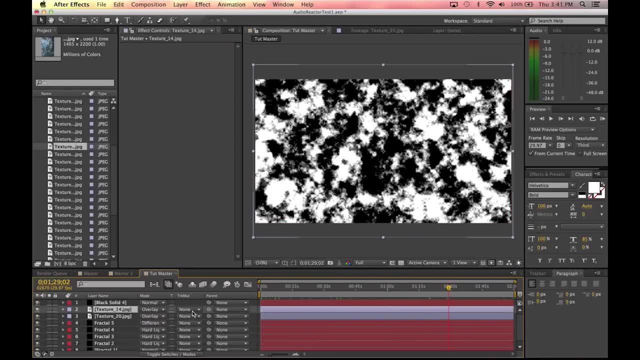 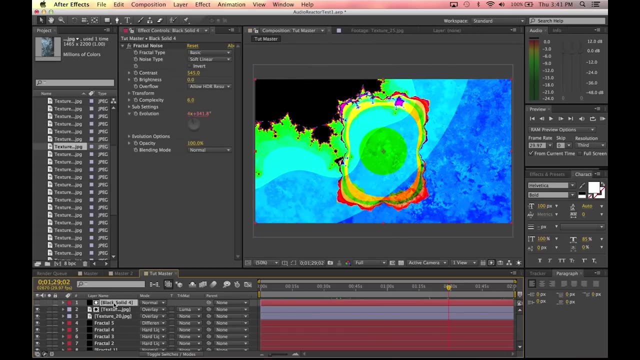 So it's changing pretty quickly here. And now what you can do. I'm going to scroll down this layer. There we go. If you change the track matte of this guy To luma matte, So it's going to take the black and white values of the layer above. 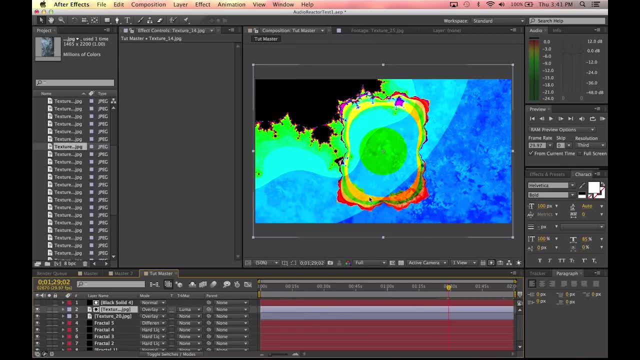 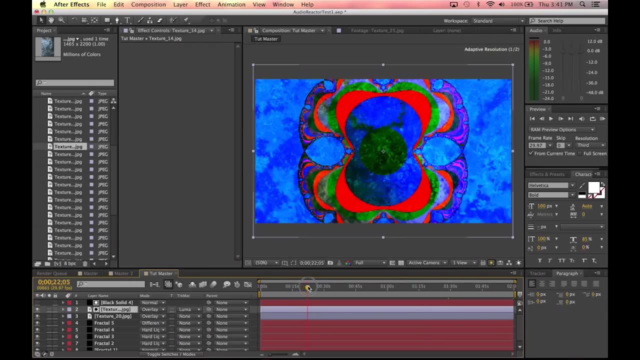 And wherever it's white, that texture will appear. Wherever it's black, the texture below it will appear. So the textures are going to be changing in the background. now, This is something I didn't do in the example, which I probably should have. 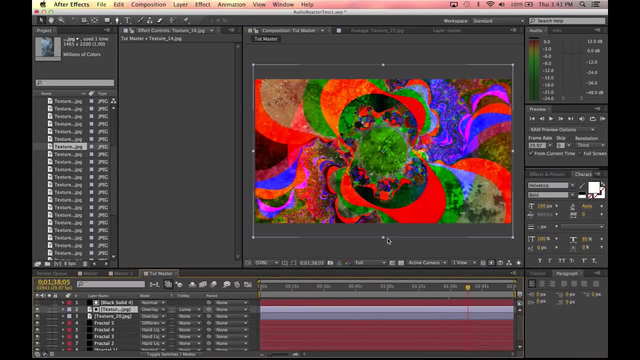 Yeah, There you go. It might be hard for you guys to see just because I'm scrolling through, But you get some really strange effects with the textures kind of blending, And I like it. It looks fractally, I guess. So I mean we're going to add some color correction. 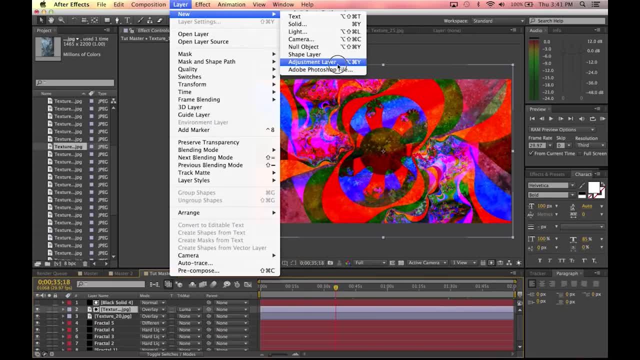 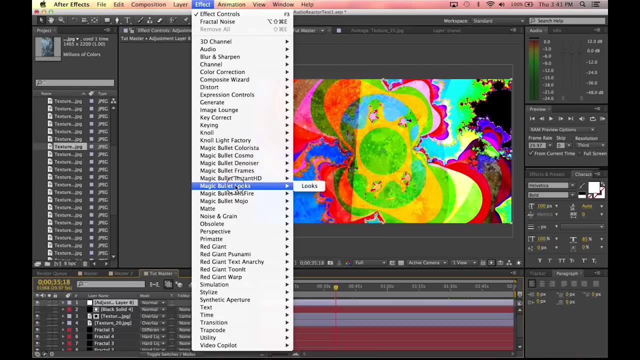 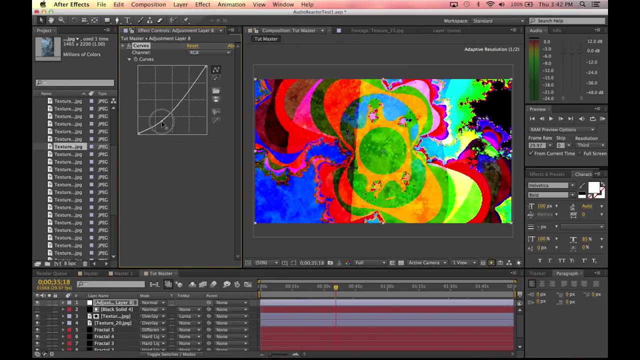 I mean, what's After Effects without color correction? So layer, new adjustment layer. All right, We're going to go to effects And I like using magic bullet looks, But because most of you guys probably don't have that, I'm just going to do color correction curves. 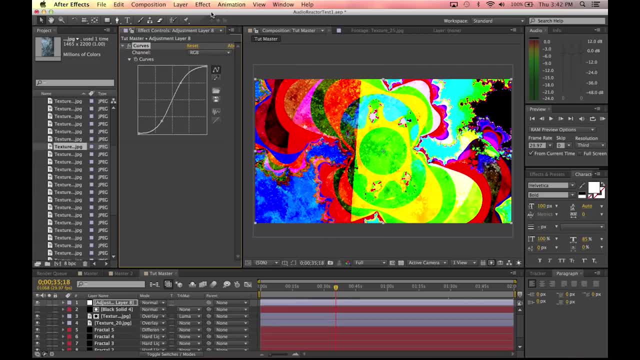 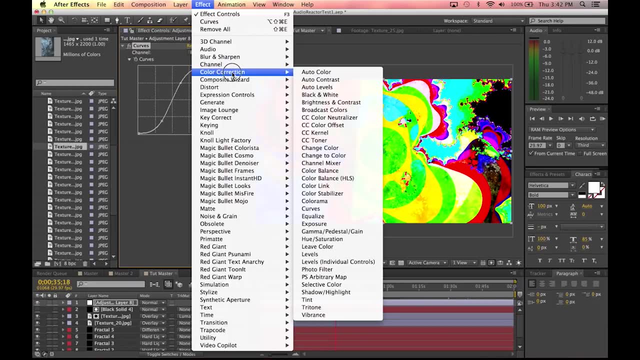 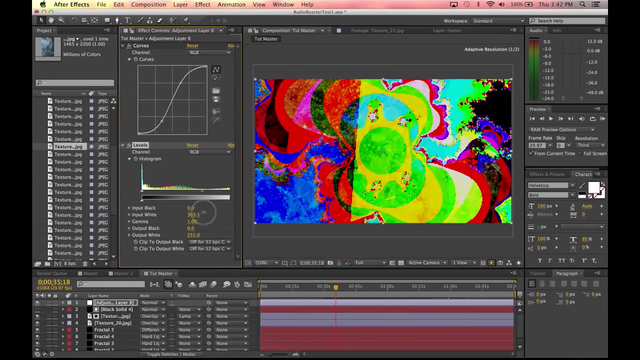 And just increase the contrast here, just to make it a little bit more dynamic. Stuff will change faster. Let's do effect. Change the levels a little bit, Pull in the whites here, Increase the gamma, just so you can see more. I like that. 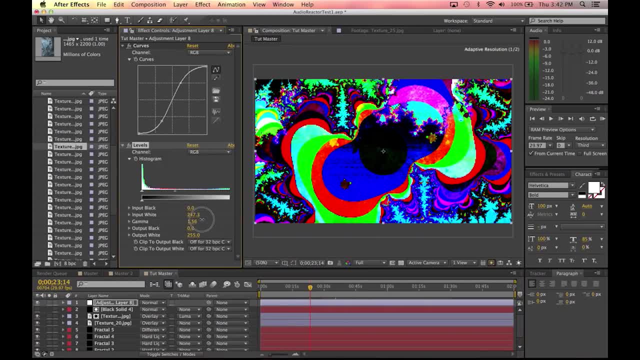 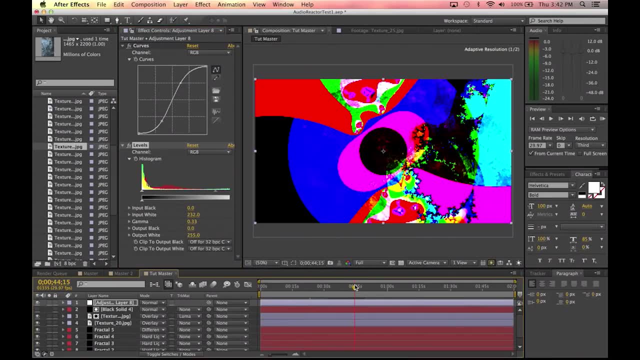 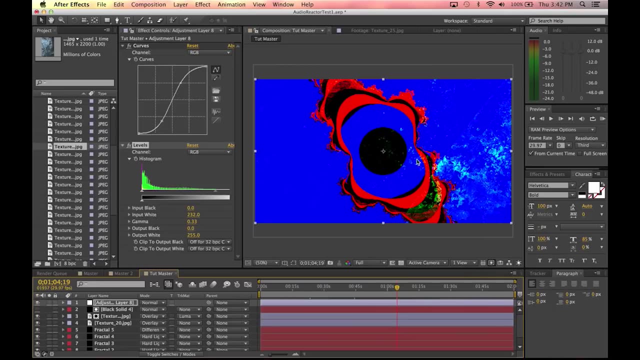 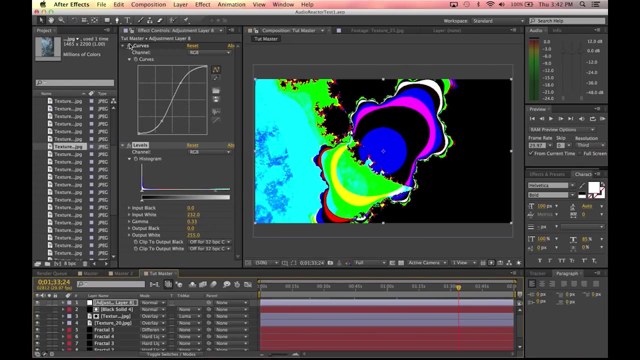 Oh, maybe too much. A little bit too bright here, Yeah, but when working with abstract stuff like this, you really don't need to follow all the rules. So, all right, I like that. OK, I'm going to save it. 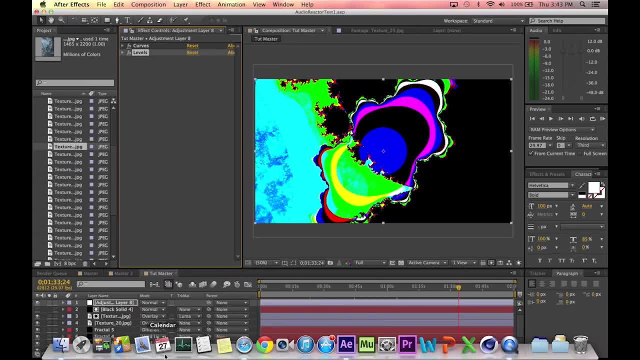 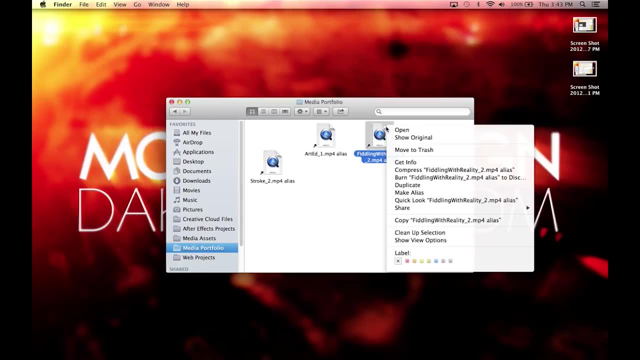 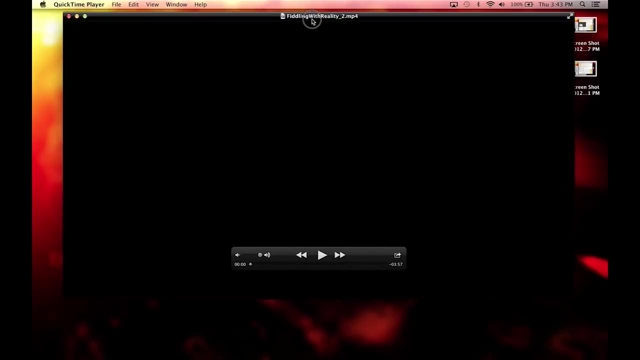 All right. And now, if we go back to the original example, let's see I have that under quick time here, All right, Actually I'm recording on quick time, So hopefully this doesn't mess up things. We'll see. 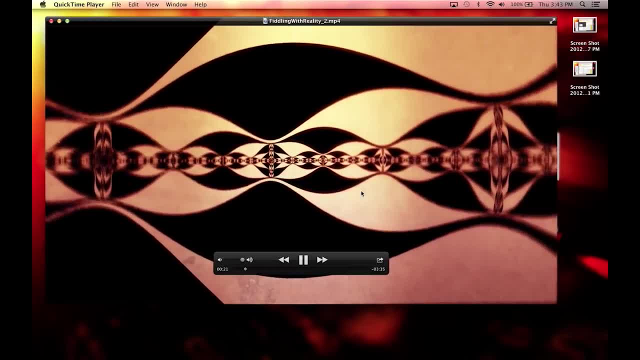 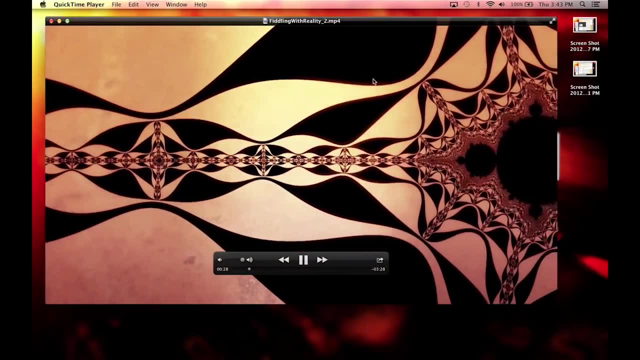 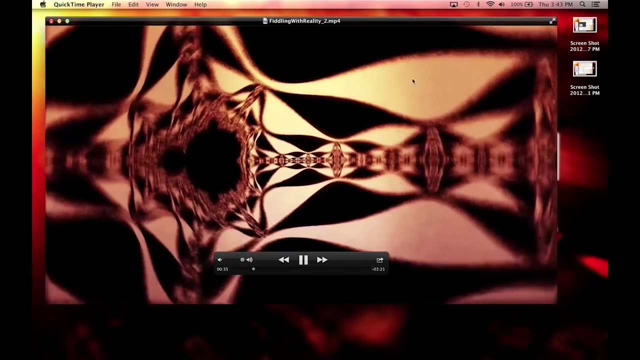 So you can see at the beginning here. hopefully you guys can hear the audio. But as this bass drum kicks in, the whole animation is kind of fluctuating with those values. So when the bass drum gets real loud it really blurs the scene. 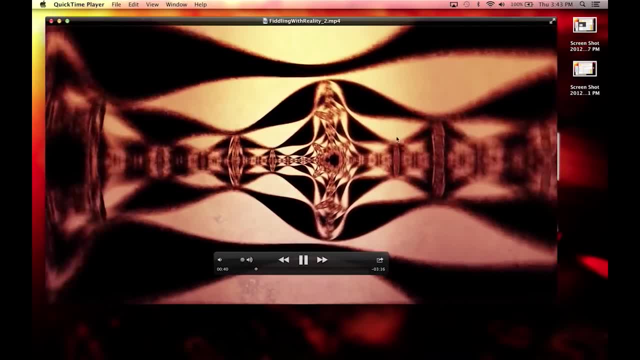 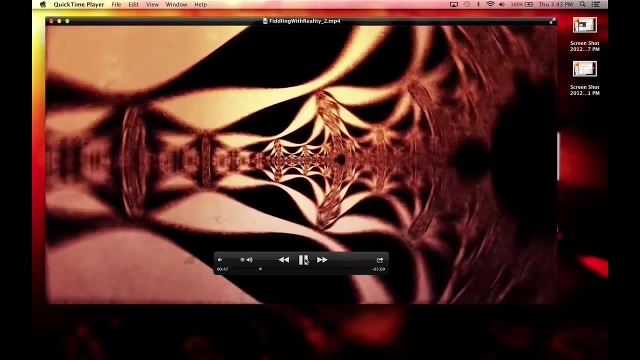 I really like this effect. You can use it with all sorts of things. I mean you can link the audio values to any value in After Effects. Very powerful: creating animation with very few key frames. So I'm going to show you guys how to do that real quick here. 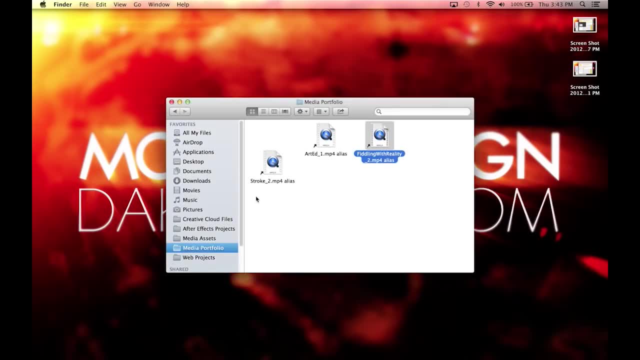 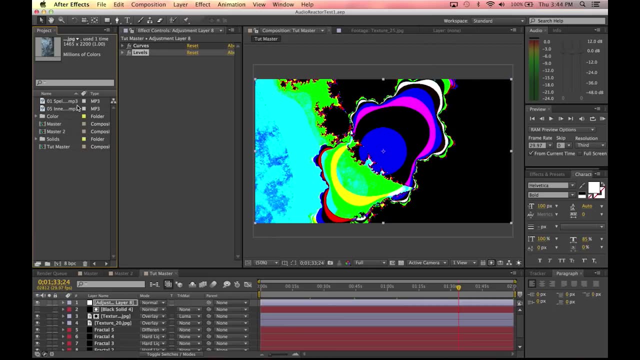 In fact, I think the next tutorial might be on something similar. You guys will see I'm going to go back to After Effects here. Here we go. Let's see. The music I'm using, by the way, is called Spellbound. 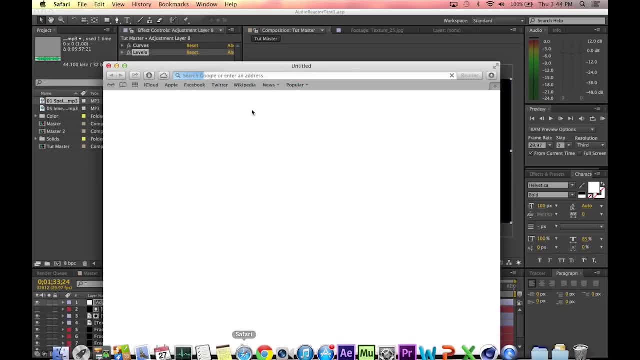 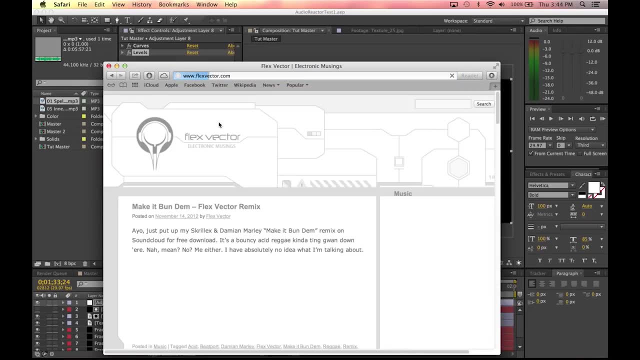 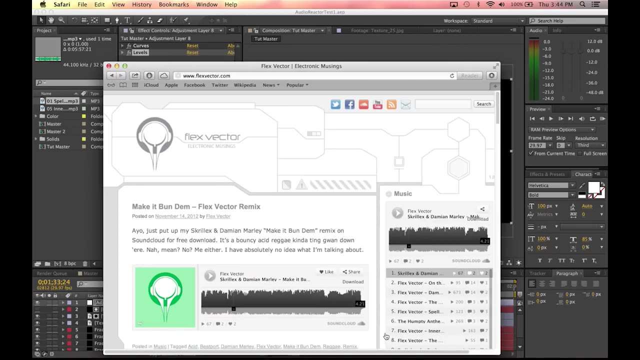 It's called Spellbound, Spellbound from this guy named calls himself FlexVector. Let me just pull up his website here: flexvectorcom. There's a link to it on the blog. Excuse me, Anyways, he has some really strange music, but very, very interesting. 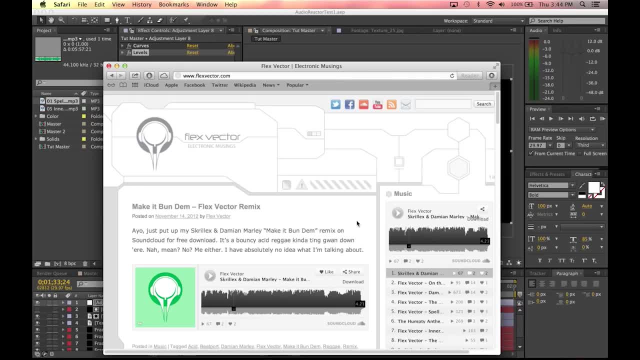 I like it a lot. Also, his music is Creative Commons, so you guys can use it for basically whatever you want, as long as you're not selling it. I contacted him and asked him if it was cool if I used his music in my animation. 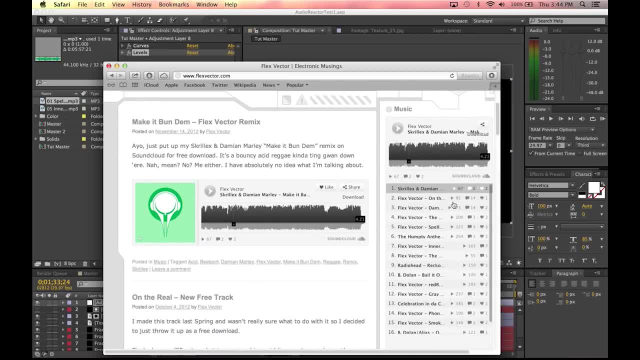 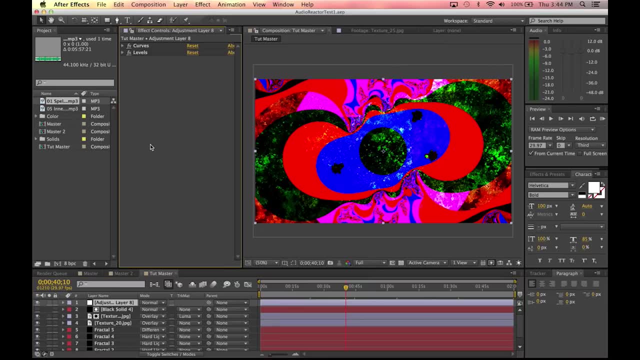 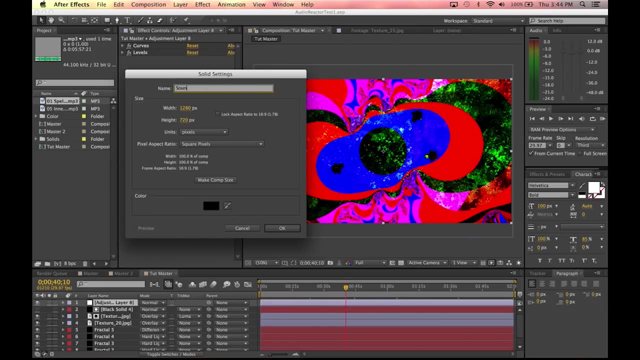 but technically you don't need to do that since it is Creative Commons. He's a really cool guy. I recommend his music. All right, so what are we going to do? Oh yeah, All right, layer, new solid and we're going to call this sound keys. 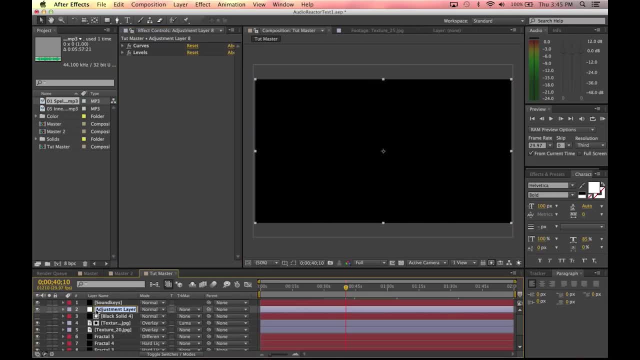 Let me just rename this layer below adjustment layer. We're going to call it color Color correction. Whoops, put three Rs, but that's okay, All right, Just to keep our layers in order here. All right, so sound keys. 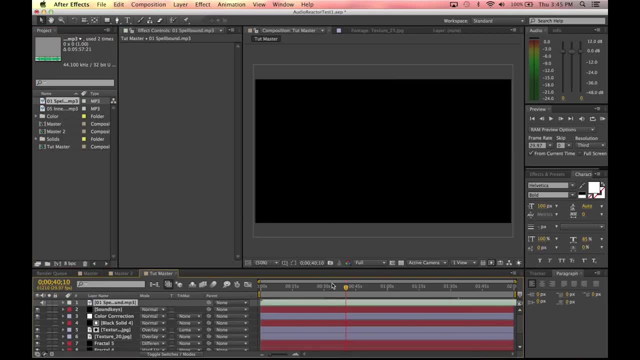 I've got to pull in the audio file here. I'm going to use the same song. Actually, I'm going to use a different song. It's a little bit more dynamic. There we go. All right, delete that. It doesn't matter what song you use. 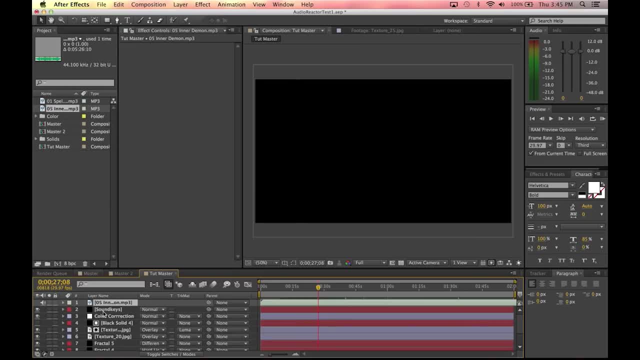 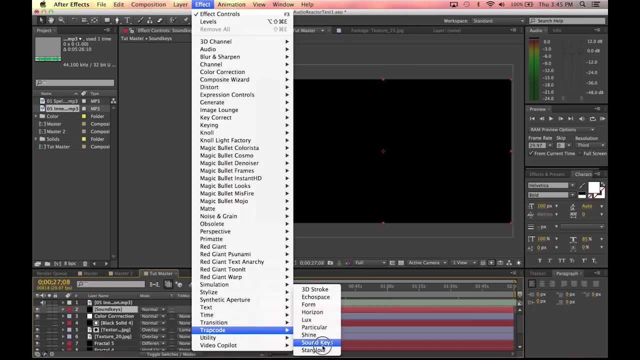 I mean, obviously it's up to you. Okay, So we don't see anything because that's our black layer here. So we're going to click on that layer, Go to effect trap code and sorry, not everybody will have this plug-in. 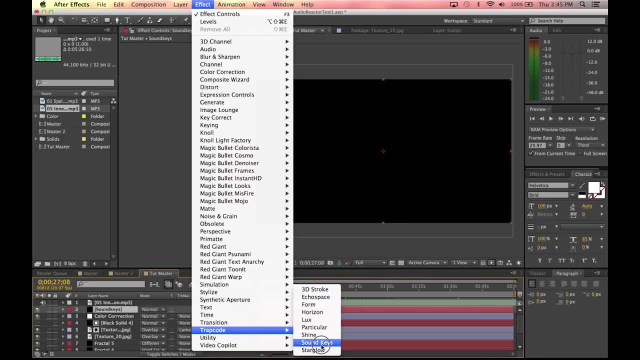 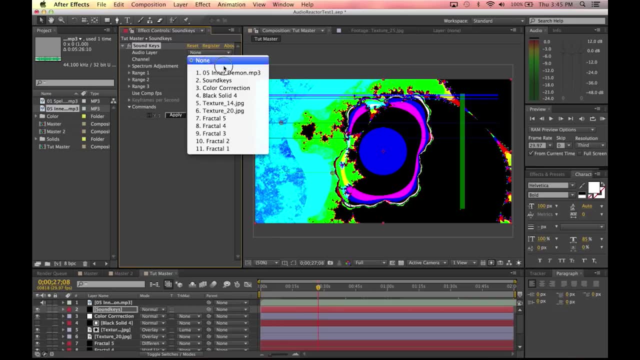 You have to buy it from Red Giant. So for those of you that do have it, great If you don't, that's all right, It doesn't really matter, It's just an extra effect. You can still get the fractal animation going. 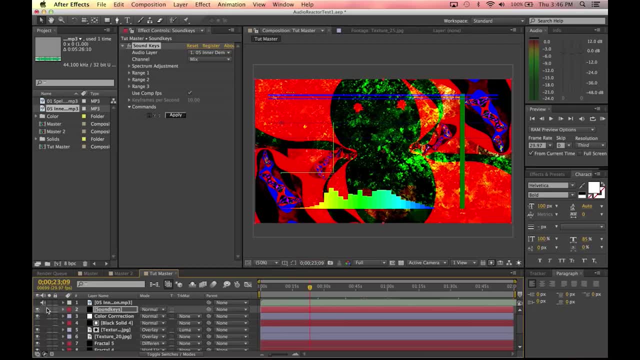 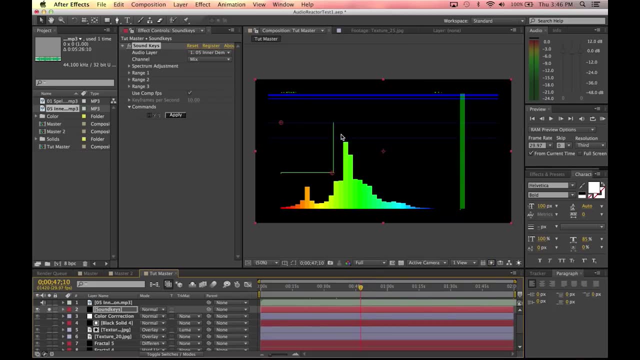 So here we go. So let me just swallow this layer, All right, So you can see the values here. This one goes really high, So I'm going to change the range. Also, if there's any Red Giant developers listening to this by chance, 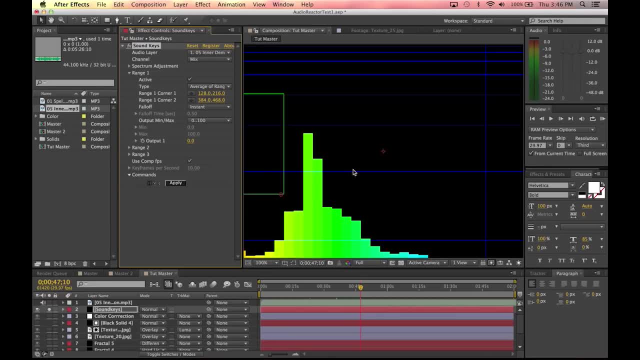 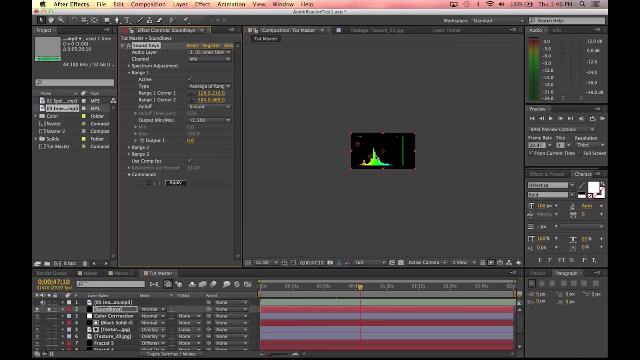 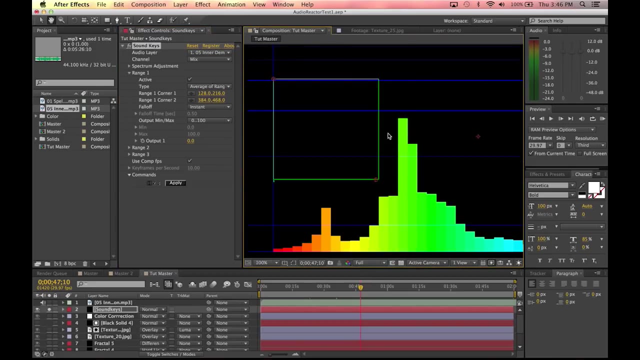 there's a problem with the retina displays. I'm using a retina display MacBook. This line here is one pixel, So if I scroll out I cannot see the line at all and it's pretty annoying. So hopefully somebody figures out how to fix that. 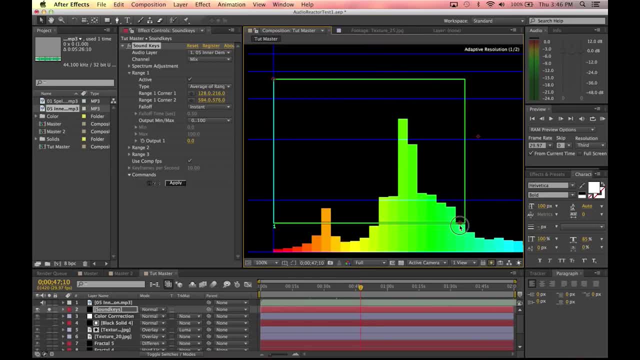 All right, I'm just going to isolate these values here, And so, basically, what SoundKeys does is it analyzes your audio And, however, I think it goes by like percentage that this box is filled by the waveform. If it's all the way full, it's going to be a percentage of 100%, obviously. 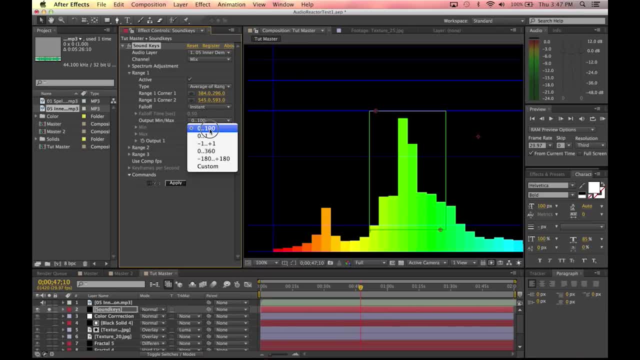 And it's going to output a value which you can change. It could output, you know, 100% will be 360.. Or 100% will be 1 or 100. For this one, we're going to use 100.. 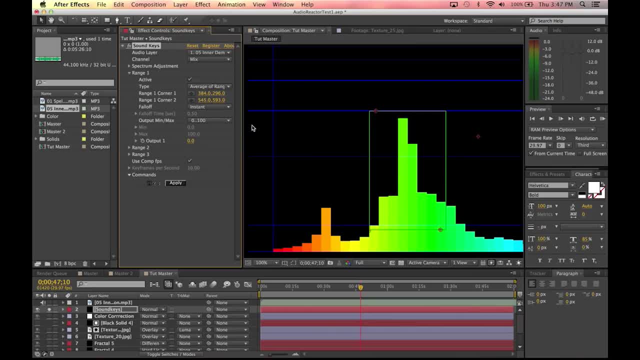 And so if it's 50% full, it's going to output a value of 50 in a keyframe, which is really useful as you'll see later. So we're just going to use one value. I mean, you could keyframe all sorts of stuff and have them doing all sorts of different things. 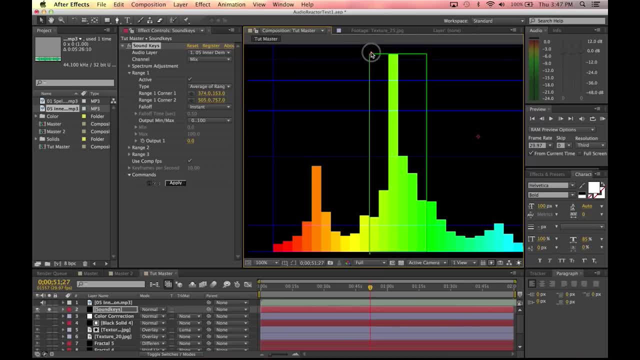 I'm actually going to keyframe the entire thing here And you'll see why later. All right, There we go And I'm going to click Apply. So that's going to take a while here. It's going to analyze the music and render out all of these keyframes. 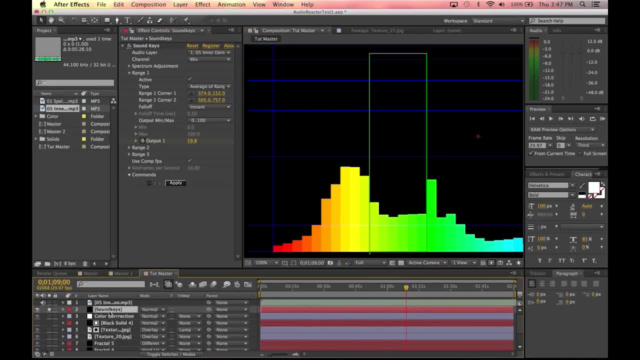 all of these values for the entire length of the song And if you click on the value and press U, you can see hundreds and hundreds and hundreds of keyframes. And the value down here right now is at 20.. It fluctuates. 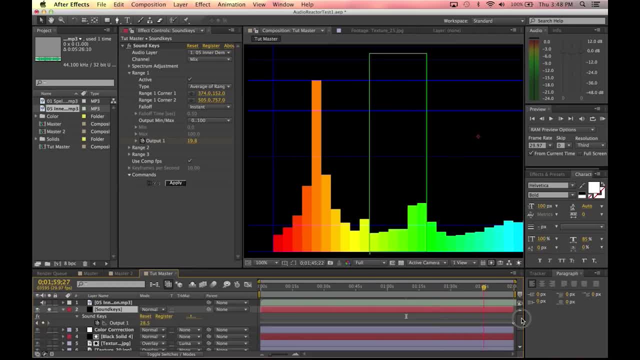 And it's good to realize what values. It looks like we're not really going too high. We're not too high above 30. It looks like 37 was the highest I saw, So about 40 is going to be our limit. 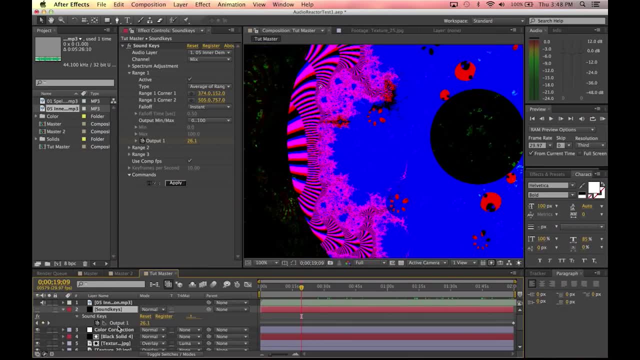 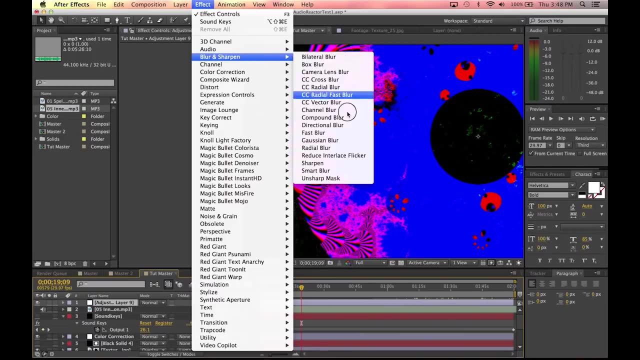 All right, We're actually going to turn off this layer, so we don't need it. All we need is those keyframe values. Now, if you do Layer New Adjustment Layer, I like using Radial Blur, It gets some really cool effects. 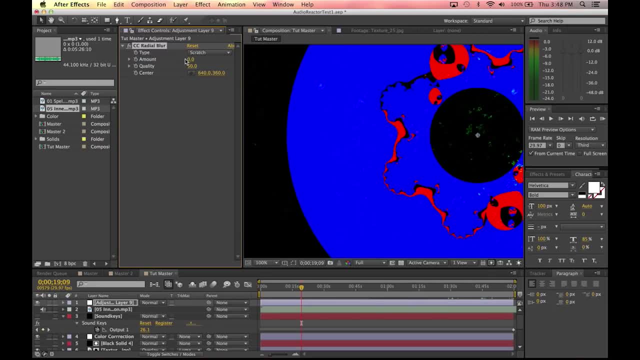 But I'm warning you guys, it's going to render very, very slow, So be careful, Don't crank this value up too high, Otherwise it could take, I mean, several minutes to render. So, anyways, I'm going to animate this value. 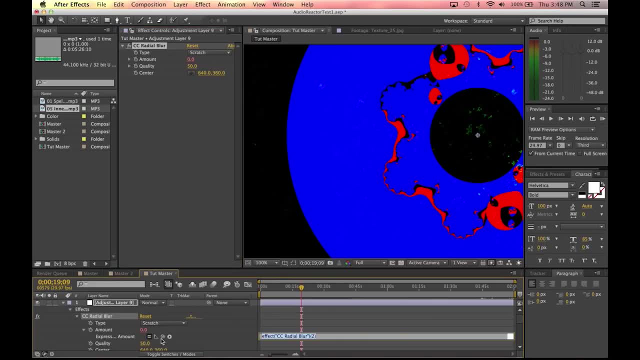 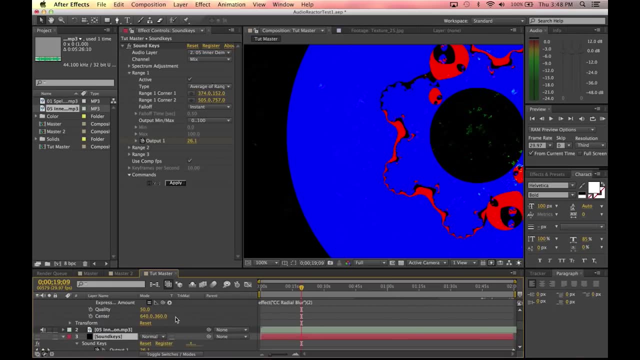 We're going to Alt-click on this value. That's going to bring up our stopwatch here. Going to go to Sound Keys Layer. We're going to pick whip And we're going to add this value to the output of that layer. So it's going to basically say: okay, trap code: sound keys is rendering a value of 26.. 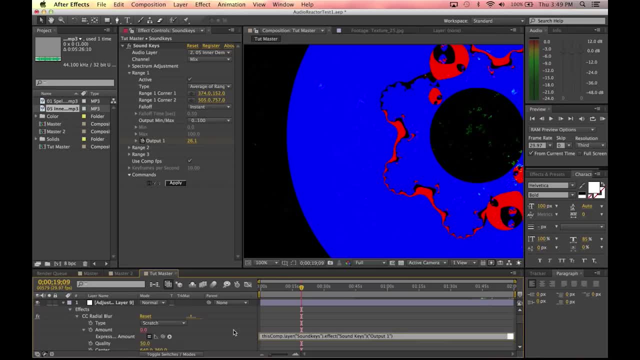 So that means I'm going to use a blur value of 26. And of course that's really high. So what we can do: if you click on this layer again, go into the keyframes and I'm going to add parentheses at the end. 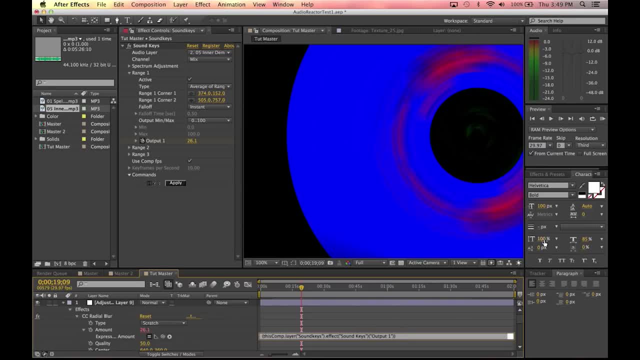 Parentheses at the beginning. So it's. I mean just simple math here. The value right now is 26.. I want it to be, I don't know, closer to 5 maybe. So if you say minus 5.. 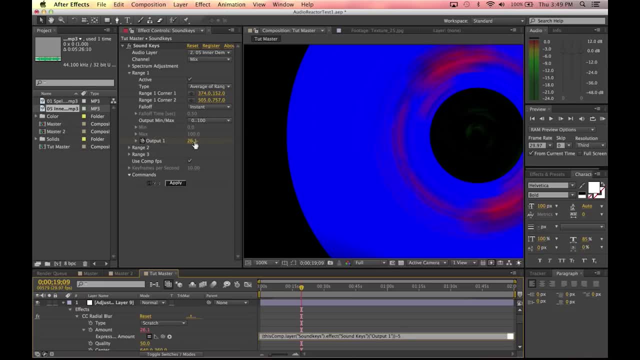 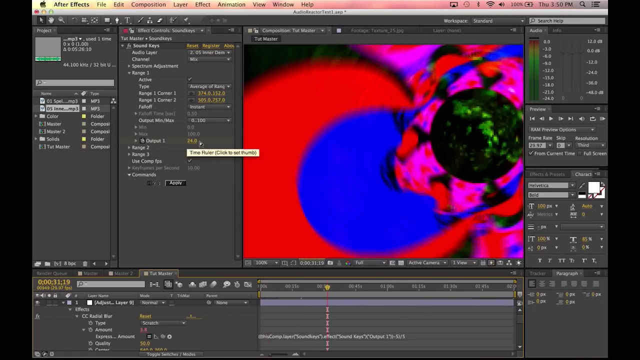 So now it's going to say 26,. right, Minus 5. It's going to be 21.. And now you can add another parentheses Divided by backslash, here 5.. So now it's going to say any value that we get, we're going to subtract 5 from it first. 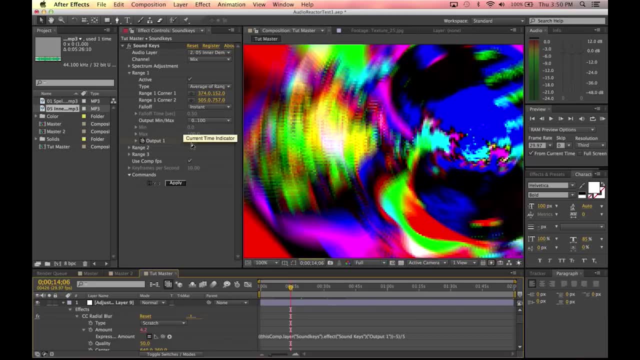 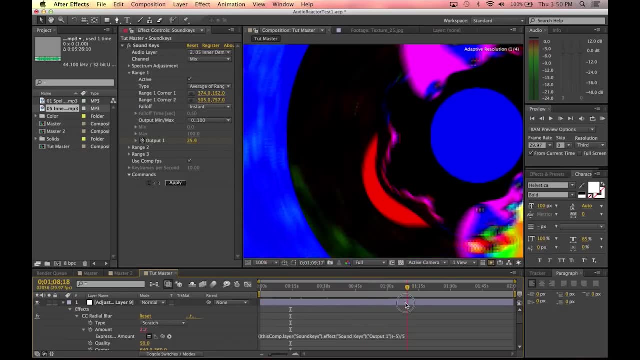 So if it was 0, then you're going to get a value of negative 5.. And then it's going to divide it by 5. So that's going to get you negative 1.. If it was 20, it's going to subtract 5, right? 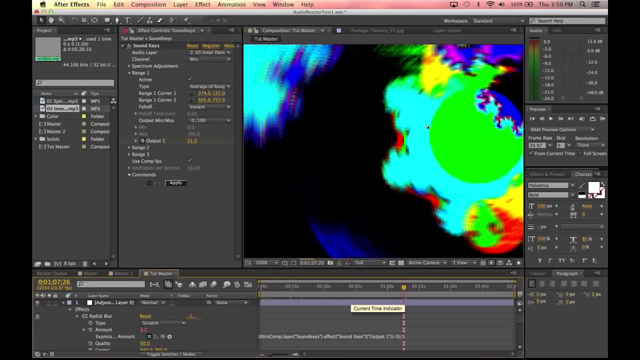 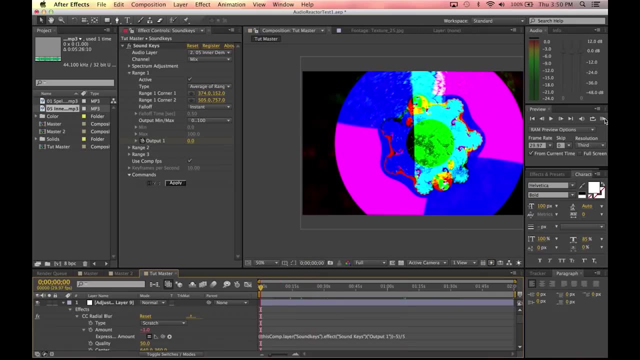 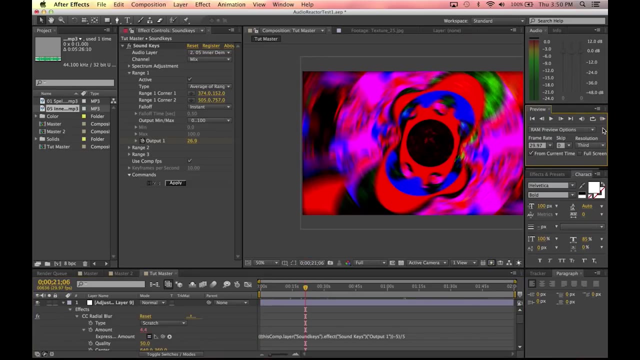 And then divide it by 5. It's basically lowering the values into a more usable range. But as we render here, let me do a quick RAM preview. Actually skip forward in the timeline. so something's happening. RAM preview here And again. it's going to take a while to render because this is a blur effect. 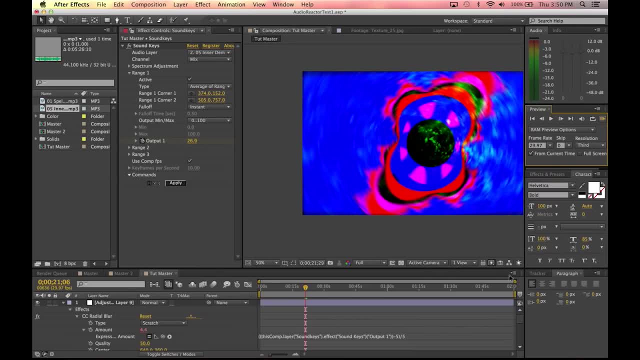 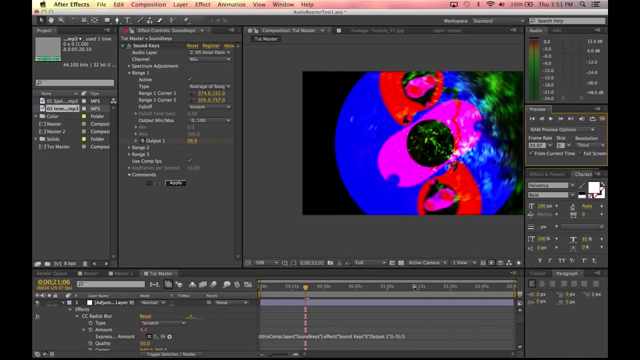 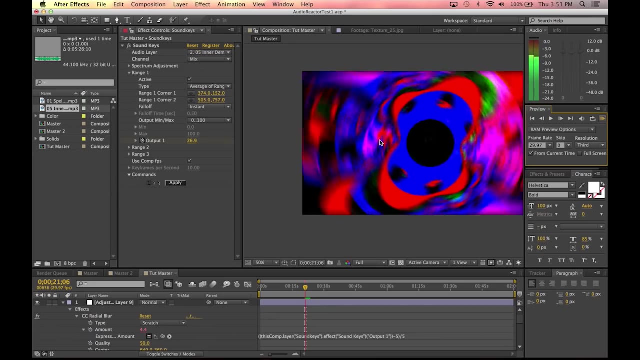 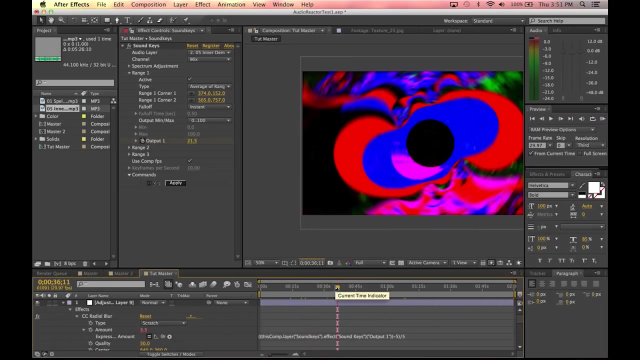 Sorry, not a very interesting video. All right, So I don't know if you guys can hear it, but the values are fluctuating. The blur values are fluctuating with the music. Very strange song, Another one by FlexVector. All right, 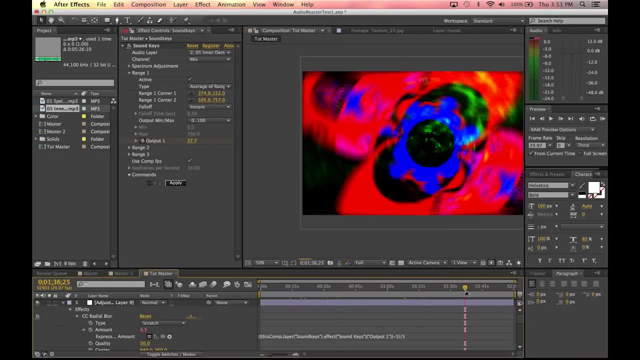 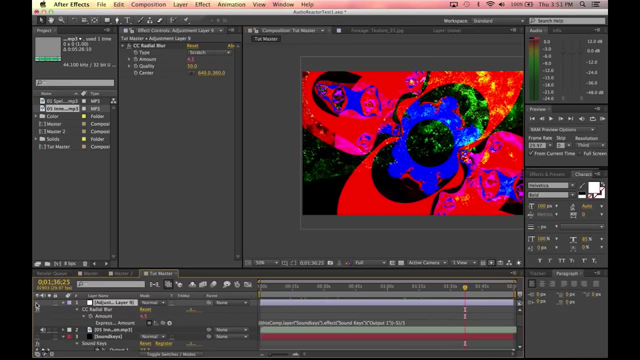 I think that's it. Yeah, I actually don't like this blur, but it turned out better on my other animation. I just used it at the beginning, so I like it with that. on this one, We could actually divide this value by 10 even. 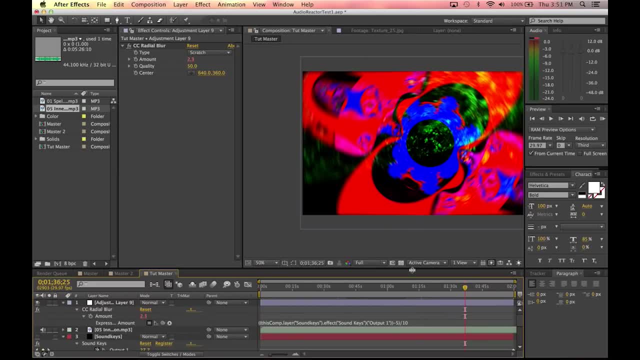 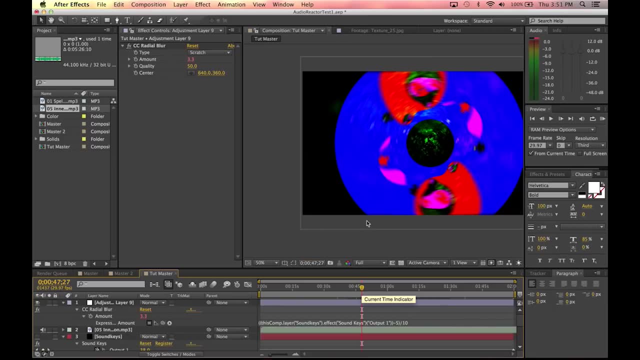 And you can see that makes it a lot more crisp, clear. Yeah, Yeah, That makes it better. All right, I think that about wraps up this tutorial. If you guys have any ideas for new tutorials, why don't you just send me an email? 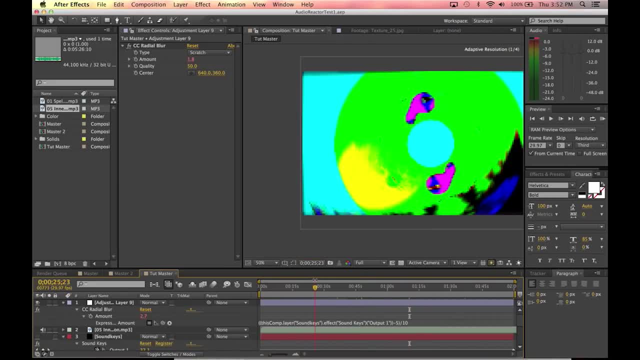 Click on contacts and allthingsmotionnet and you should be able to find me. And, yeah, Hopefully you guys like it. So have a good one.